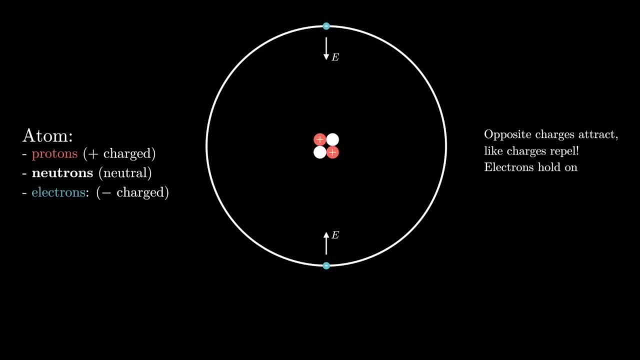 For starters, neutrons are neutral, so they don't feel electrical attraction in the first place. And if anything, protons should be repelling each other because they have equal electric charges And gravity is not strong enough to overcome that repulsion. So what's going on? How do protons and 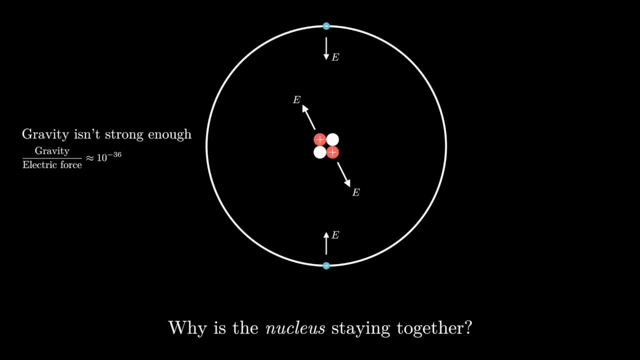 neutrons stay together. From this simple observation, we can conclude that there must be another force, A force strong enough to be able to repel neutrons, And that force is the force that holds the nucleus together. It's stronger than electromagnetism and gravity, And this force is 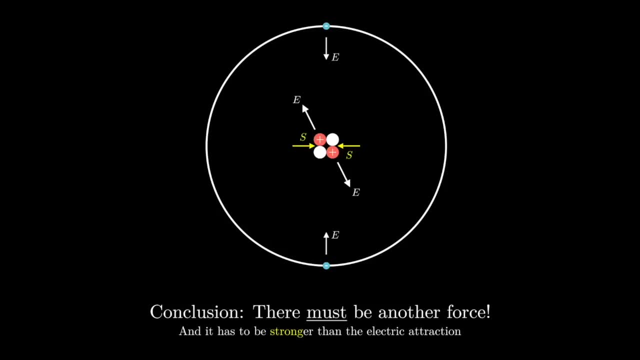 what's holding the nucleus together? At this point, we know virtually nothing about this force, except that it must be really strong. So let's call it the strong force, which is exactly what physicists did in the 1950s. To solve the mystery of the strong force, physicists started building the 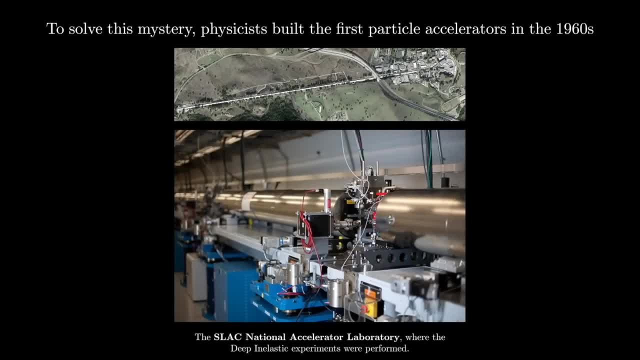 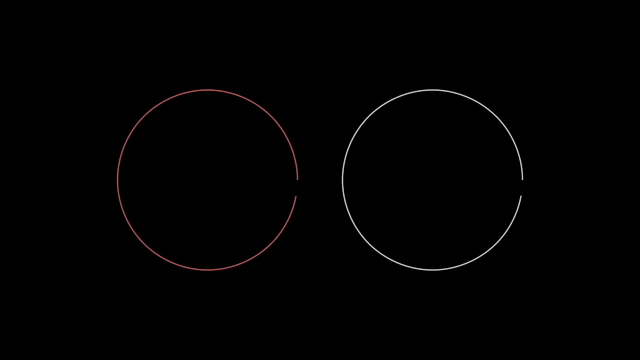 first particle accelerators in the 1960s, And the experiments they designed using those accelerators were extremely clever and beautiful. But you've seen the length of this video, I have to cut corners somewhere. So let's skip to the discoveries, because at first they made no sense. As it turns, 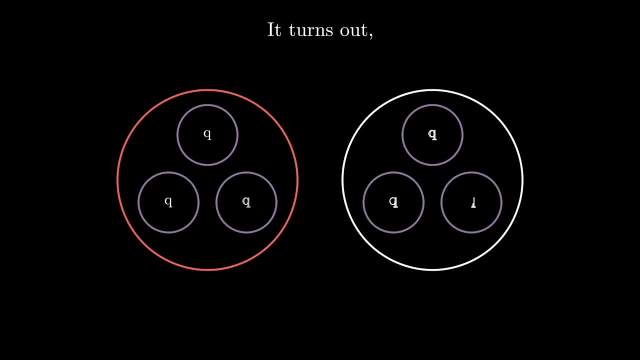 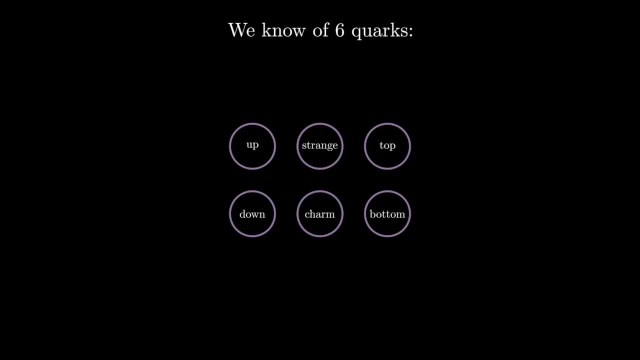 out. protons and neutrons are made of three other smaller particles known as quarks. In total, we have found six kinds of quarks and we have given them six silly names: Up down, strange charm, top And bottom, Beautiful, No notes. Protons and neutrons are made of only two of these kinds. 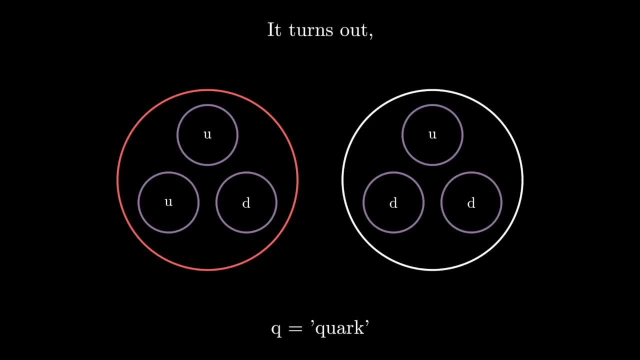 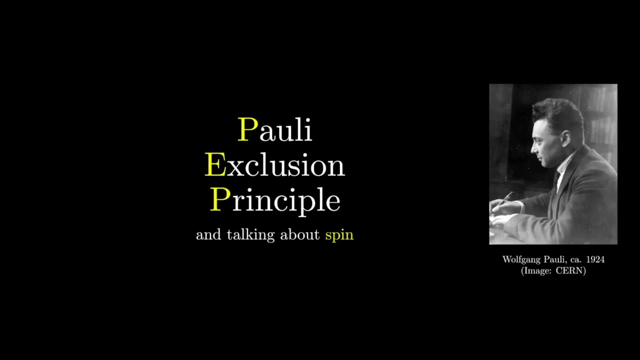 of quarks. Protons are made of two up quarks and one down quark, while neutrons are made of two down quarks and one up quark. To understand why this was so confusing at first, we have to talk about Pauli's Exclusion Principle. And to talk about Pauli's Exclusion Principle, we have to talk. 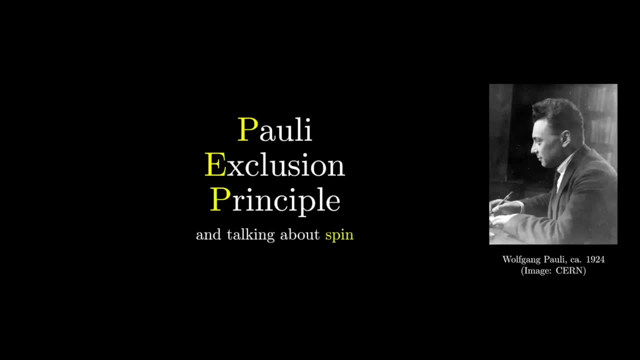 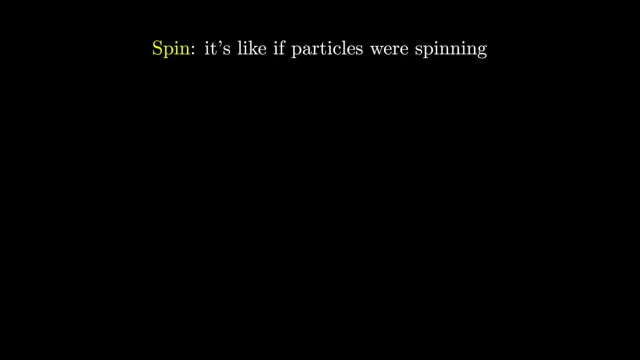 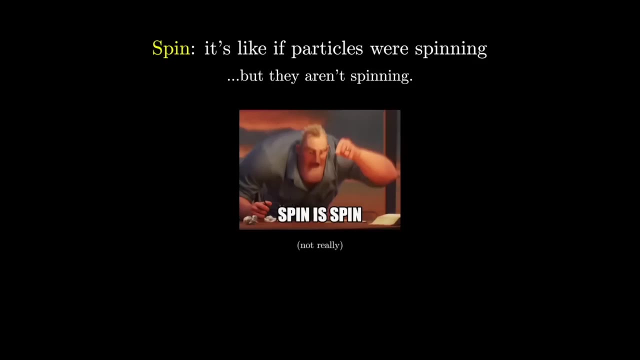 about spin, Part one, Pauli's Exclusion Principle. Spin is called spin because it's like if particles were spinning in one direction or the other. Except it's also not like that at all, because particles are point-like and points do not spin. 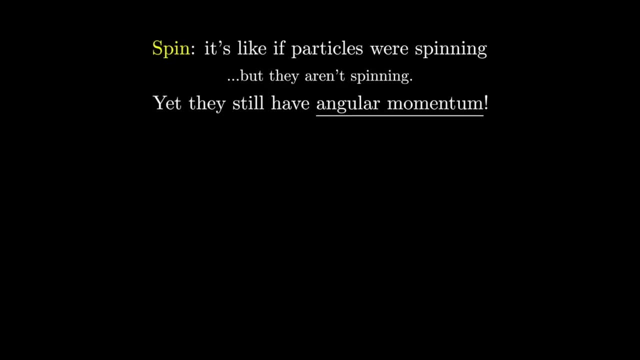 And yet they do have angular momentum. Look, the nature of spin is a really fun discussion to have, but it's also extremely complex and difficult. But thankfully, spin are actually quite easy to understand, so let's just focus on that. And if you want to learn, 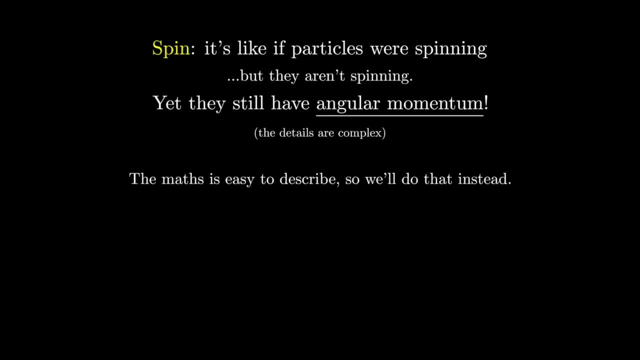 more about the nature of spin. I'm going to leave you some links in the description and I wish you the best of luck. Spin is a quantity whose value, which we call the spin quantum number, changes in steps of one unit, never going above nor below a given absolute value. 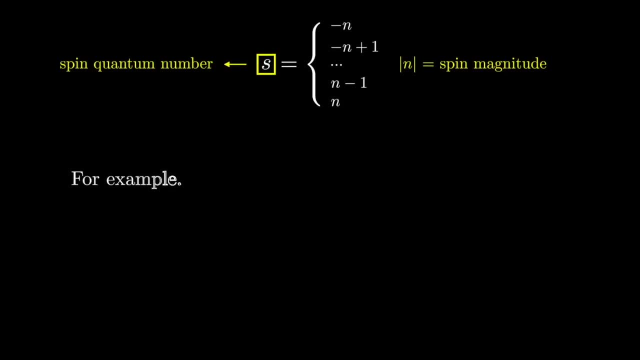 called the magnitude. For example, electrons, protons and neutrons all have spin with a magnitude of 1 1⁄2. So their allowed values are only 1 1⁄2 and minus 1 1⁄2. We call these kinds of particles. 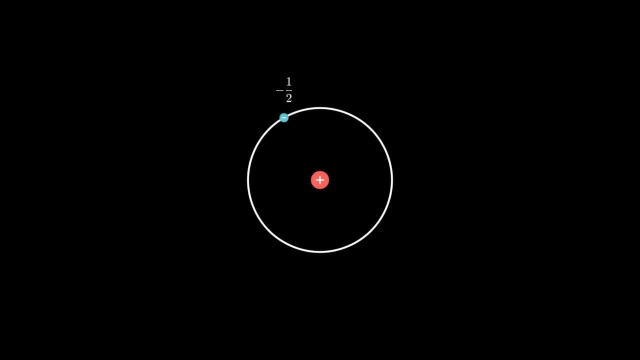 fermions. For example, let's say that we have an electron with a spin of minus 1 1⁄2, and then comes along a photon with a spin of 1. If this electron absorbs that photon, the action of the 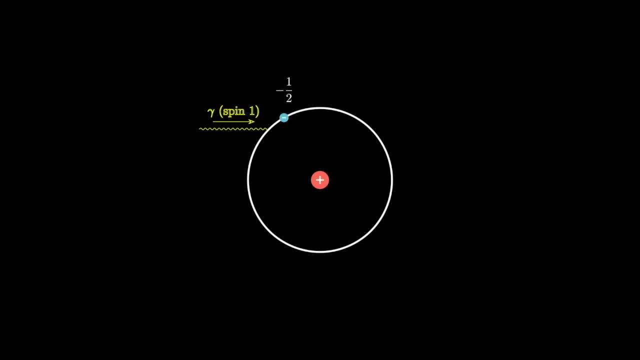 photon will be to change that spin by one unit, from minus 1 1⁄2 up to 1 1⁄2.. But now this electron cannot absorb that spin and it's going to spin by one unit, So we're going to have to change. that spin by one unit from minus 1 1⁄2 up to 1 1⁄2.. But now this electron cannot absorb that spin and it's going to spin by one unit from minus 1 1⁄2 up to 1 1⁄2.. But now this electron cannot absorb. 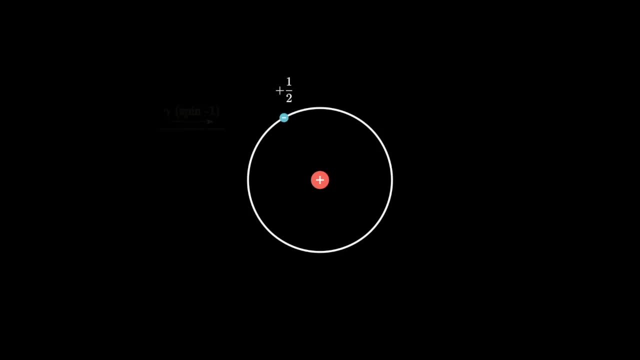 another photon with spin 1, because it cannot go above 1⁄2.. However, it can absorb a photon with spin of minus 1, going back to minus 1 1⁄2, at which point it cannot absorb another photon with. 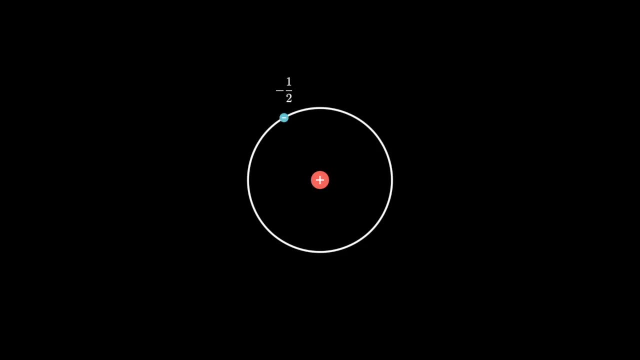 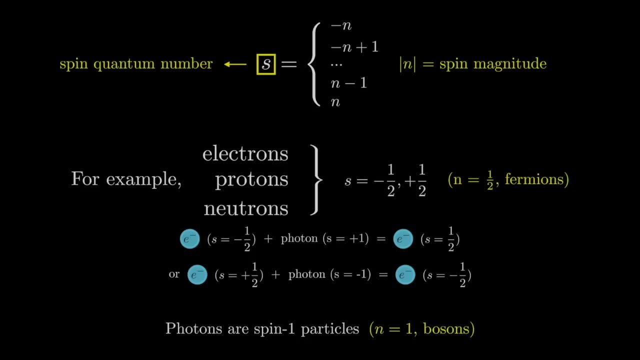 spin of minus 1, because it cannot go below minus 1 1⁄2.. As you can see from this example, photons can carry more spin than electrons, protons or neutrons, And this is because their spin magnitude is actually 1.. We call this kind of particles fermions and they are called fermions. 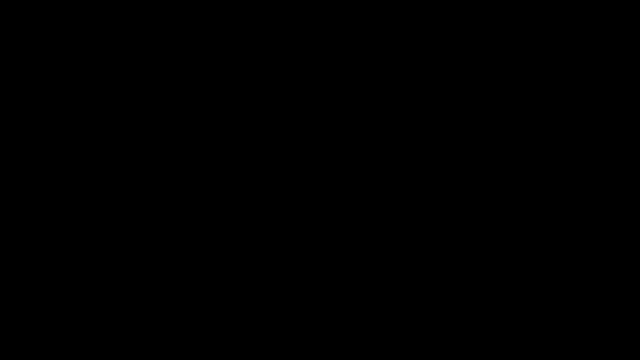 And this kind of particles with integer spin bosons. Next, because quantum mechanics is inherently probabilistic. when we measure spin, we are never quite sure which one we are going to get. We can only know the probability of getting each result. We write such probabilities using something called the wave function, For example. let's say that: 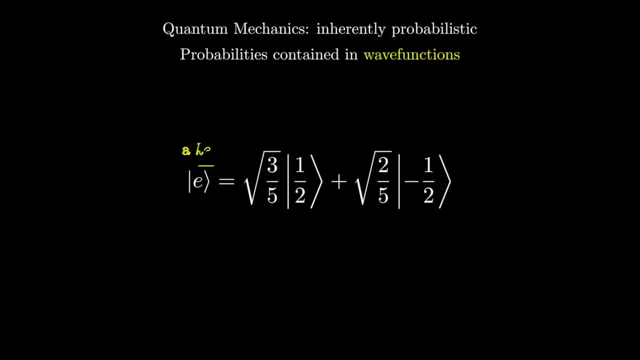 this was the wave function of an electron. This strange arrow-looking thing is called a ket. Physicists use it to specify when they are working with quantum probabilities. In this case it means that if we measure the spin of this electron, the chances of measuring a spin of 1⁄2 are of 3 in 5, or 60%, while the chances of measuring 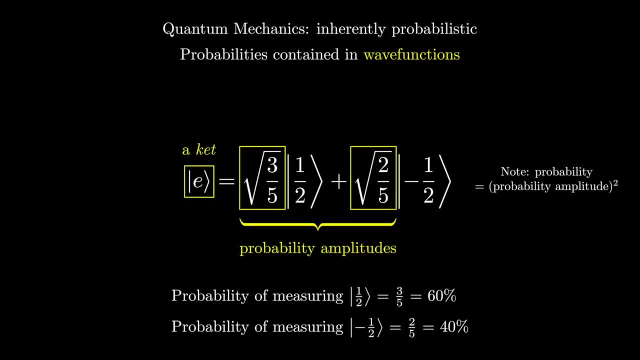 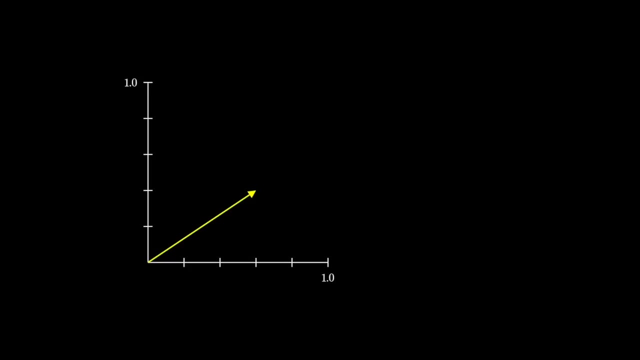 minus 1⁄2 are of 2 in 5, or 40%. Notice that the probabilities are the absolute values of the squares of each coefficient, So the coefficients themselves could be negative or even complex, and it wouldn't be an issue. We can visualize this combination of probabilities. 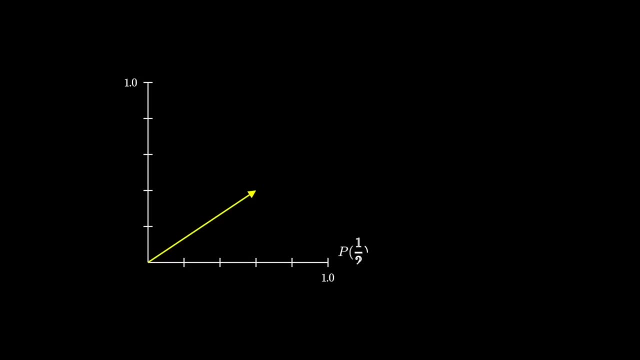 using a plane. The x-axis will be how likely you are to measure 1⁄2, and the y-axis how likely you are to measure minus 1⁄2. Now we can visualize all possible combinations of probabilities in this plane. This also means that we can think of measuring 1⁄2 as the vector 1, 0, and measuring 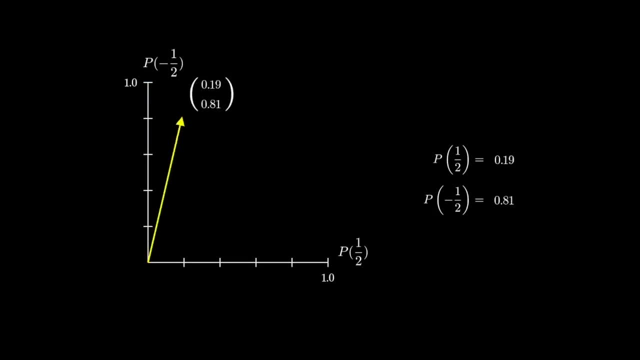 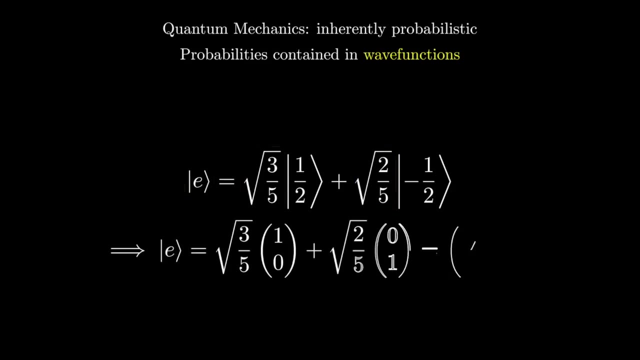 minus 1⁄2, as the vector 0, 1.. Then we can rewrite the wave function as a sum of those vectors, which means the wave function is just a vector of probabilities. This is the reason why quantum mechanics is just like spicy linear algebra. 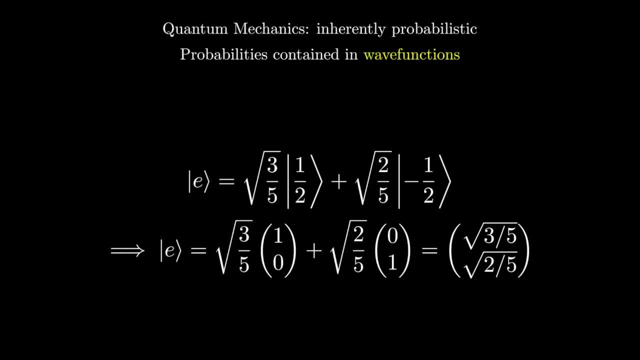 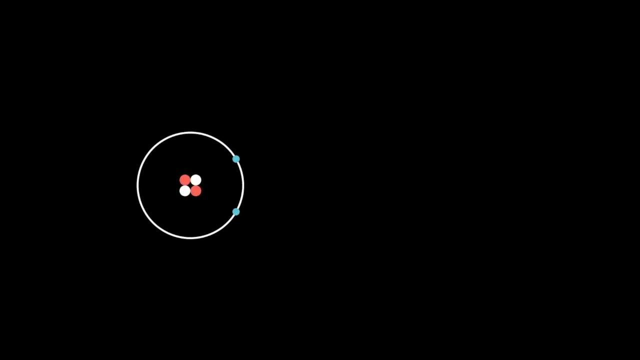 It may look like we are just finding new ways to say the same thing, and we are. That's like 80% of mathematics, But the reason we do this is because it will be very useful when we look at systems made of more than one particle, like the electrons in this helium atom. Let's call them 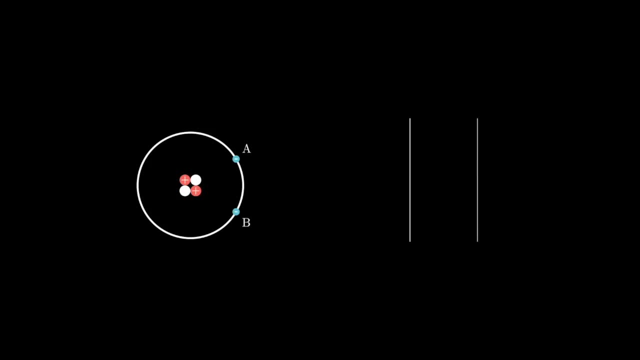 A and B. Each electron can have two values of spin, so when we measure the spin of both of them, there should be four possible outcomes, as seen in this table. What we want is to assign a vector to each outcome, just like we did before, And there are a couple of ways we could. 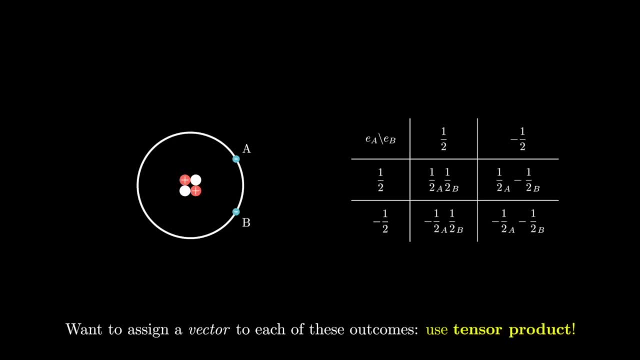 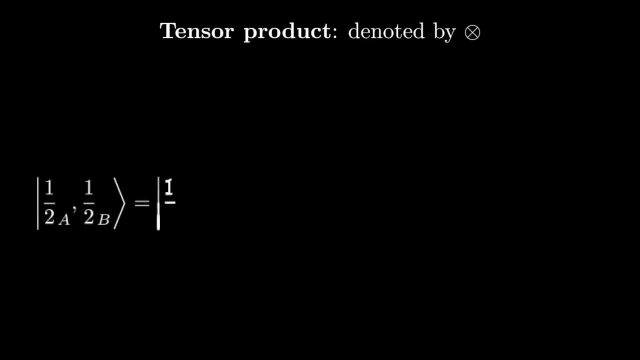 do that, But the best one is to use an operation known as the tensor product. It is a little bit hard to explain what it does with words, but it is quite easy to explain visually. Using the tensor product. we can write each outcome as a base vector. 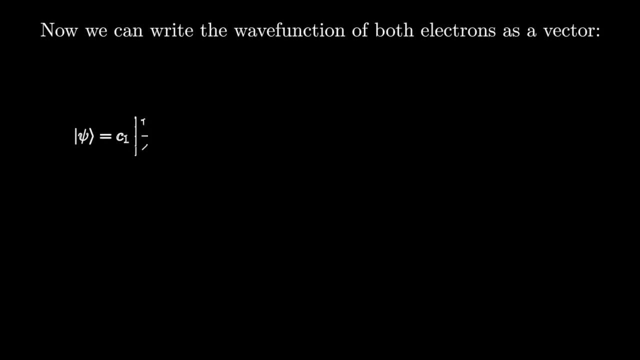 And then we can add them up to write the wave function of both electrons as a vector. We could calculate the coefficients in this vector using Schrodinger's equation, but that would be really difficult. Thankfully we don't really need to do that, All that we care. 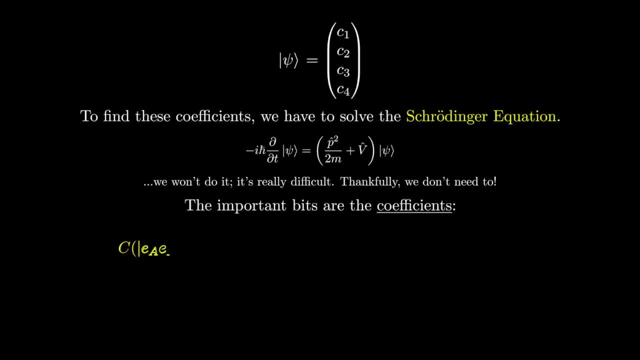 about is that the coefficients are the results of a function- Let's call it C- of A and B, And this function takes as input the function C of A and B. And this function takes as input the function C of A and B. So the lecture you just learned is actually anarc incubator. It takes as input the spin states of each. 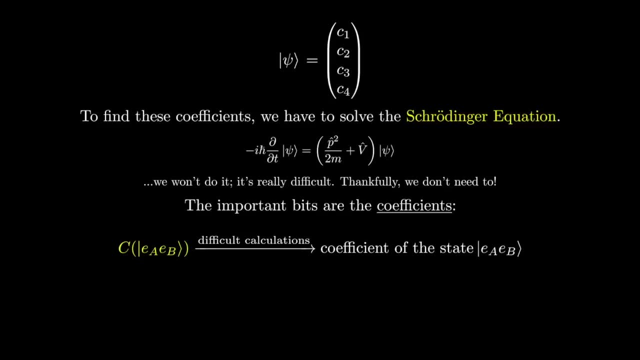 electron, And then it does whatever calculations we don't want to do to get the right results. Let me show you what this means using an example. If you give this function the inputs 1 half and minus 1 half and it outputs the square root of 1 over 4, there is a 25%. 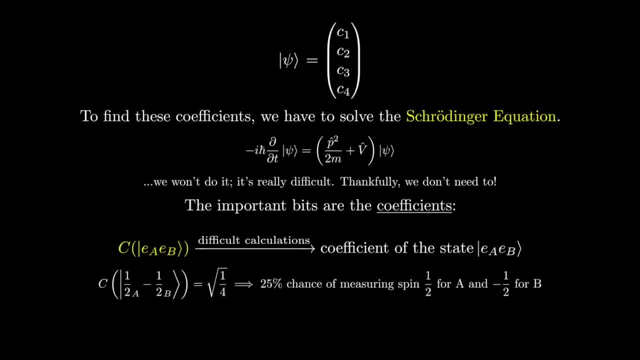 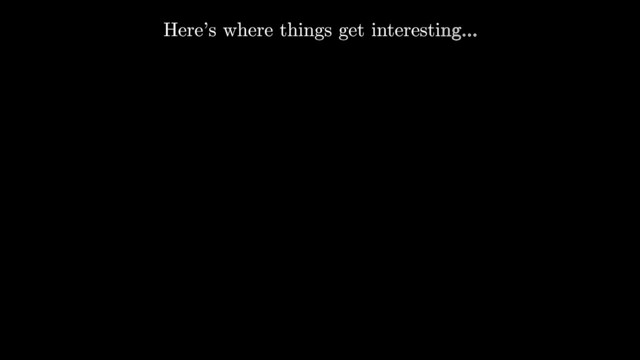 chance that you will find electron A to have a spin of one half and electron B to have a spin minus 1 half. OK, So All of that was just the background. Here is where it gets interesting. Let's go back to the tensor product. 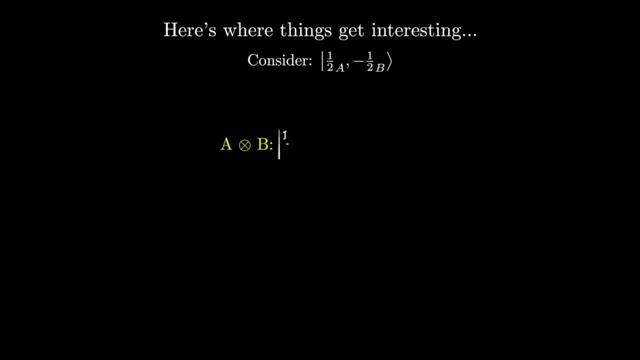 If electron A is in state one-half and electron B is in state minus one-half and we have A cross product B, then the result is the vector. But what if we had B cross product A? Then the result would be the vector. 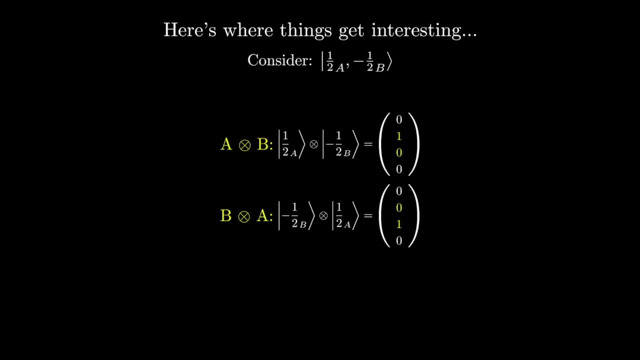 In summary, if we use A then B, we end up with one wavefunction. But if we use B then A, we end up with a slightly different wavefunction. And yet this difference shouldn't really matter. It should be like measuring distance in meters or yards- just different ways to describe. 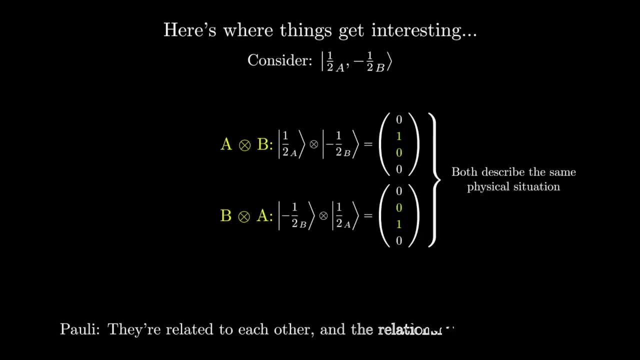 the same physical reality. Pauli wanted to know the relationship between these two different versions of the wavefunction, and what he found is that it depended on the function. If you're working with bosons, then it doesn't matter in which order you write. 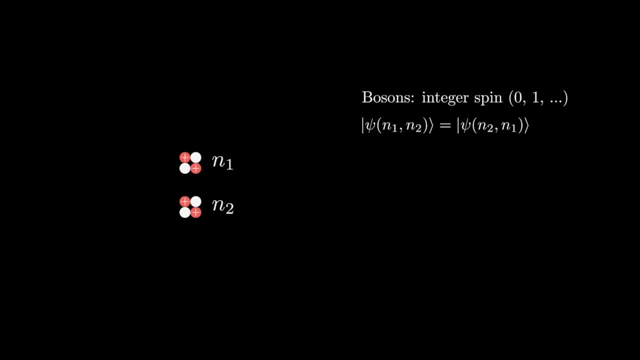 the wavefunction It will be the same either way. It is symmetric. But if you're working with fermions like we are doing right now, then the order does matter. If you switch the order of the fermions in the wavefunction, it will gain a negative. 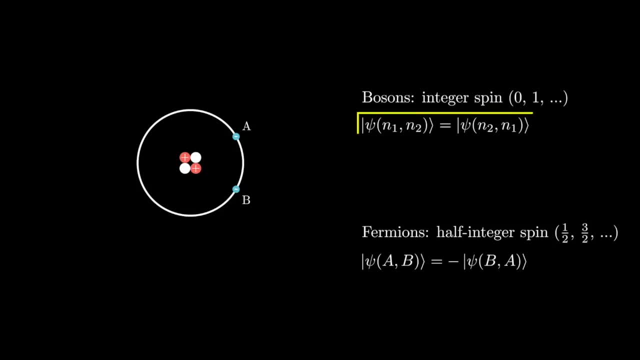 sign, It will be anti-symmetric. This is Pauli's exclusion principle And it seems complete, Completely bonkers, doesn't it? Why can't it be symmetric every time, And why does it depend on the spin? What's going on? 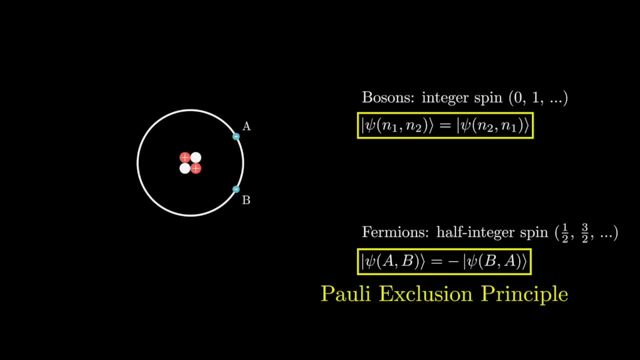 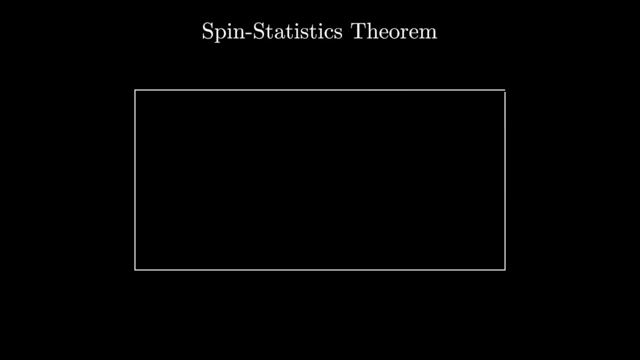 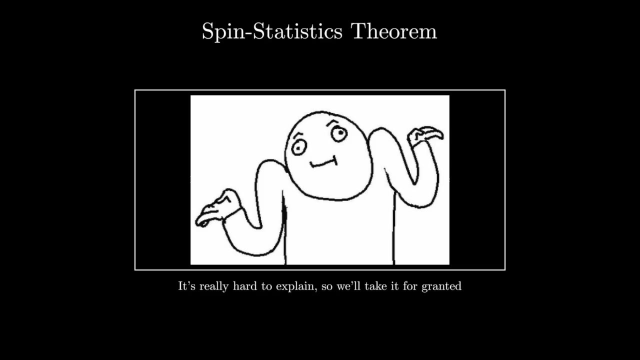 The answer lies deep in a connection between general relativity and quantum mechanics, known as the spin statistics theorem, which is really easy to explain. Here it goes. Ok, actually, it's extremely difficult to understand and to explain, and you've seen. 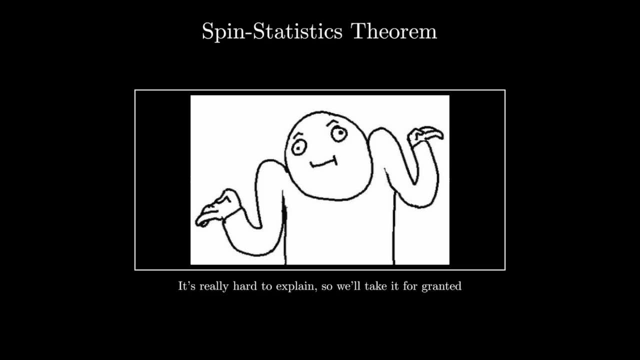 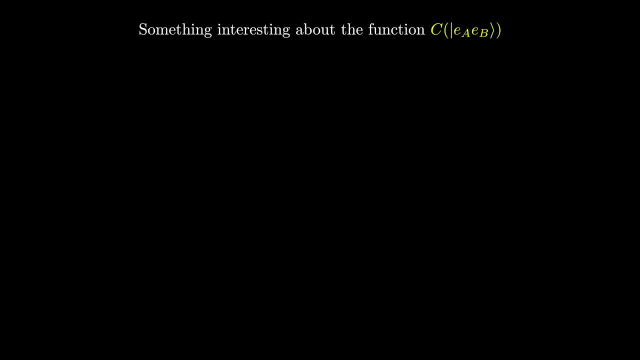 the length of this video. So let's just take it as an axiom And move on with our lives. When we look at C with this restriction in mind, we find something very interesting. C doesn't change if we switch the order of the fermions. 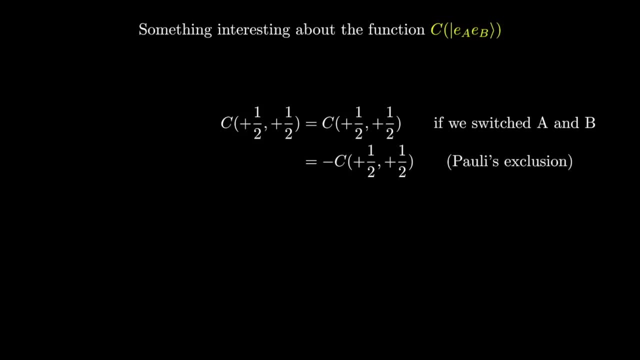 And yet Pauli demands it has to be anti-symmetric. So the only option it has is to be zero, Because only zero is equal to negative zero, Same with C. Ok, This means there is exactly 0% chance of ever measuring the same spin in both of these electrons. 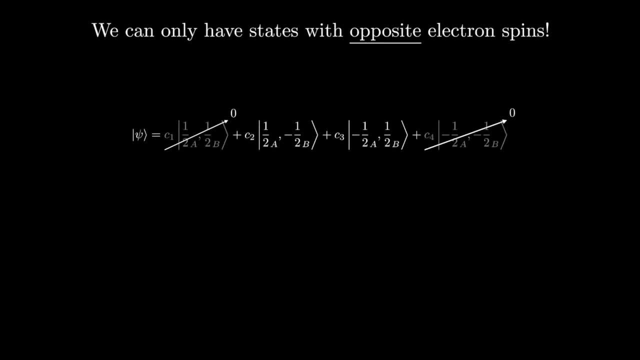 Then we are left only with the states in which the electrons have opposite spins. They must have the same coefficients but with opposite signs, And the probability must add up to 100%, which means there's always a 50% chance to measure either one. 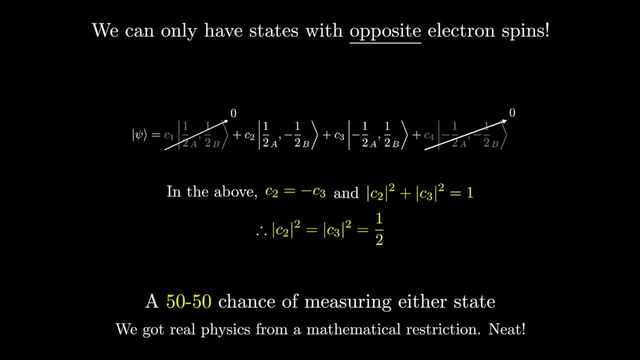 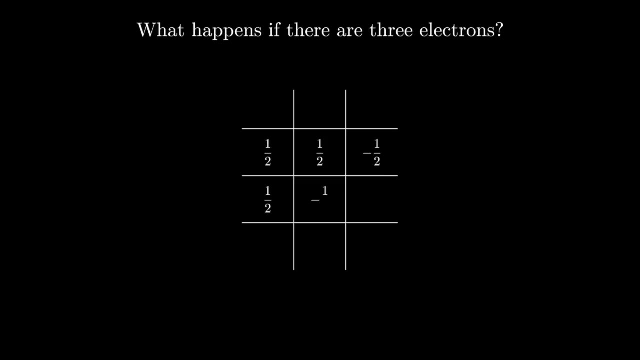 Think about what just happened. Ok, This restriction about the tensor product led us to discover real physics. Isn't that just lovely. But what happens if we have three electrons instead of only two? Because now, no matter what, at least two electrons will have the same spin. 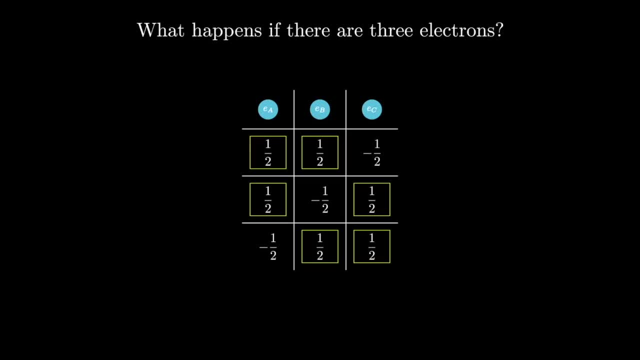 I mean there are only two possibilities and three particles. At least two of them have to share. This is not anti-symmetric, because we could switch the two electrons with the same spin and the wavefunction would be the same. Ok. 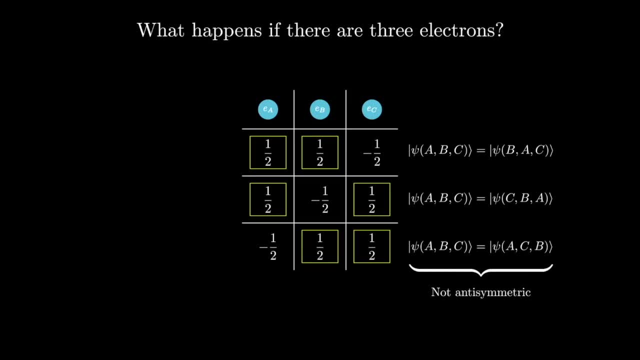 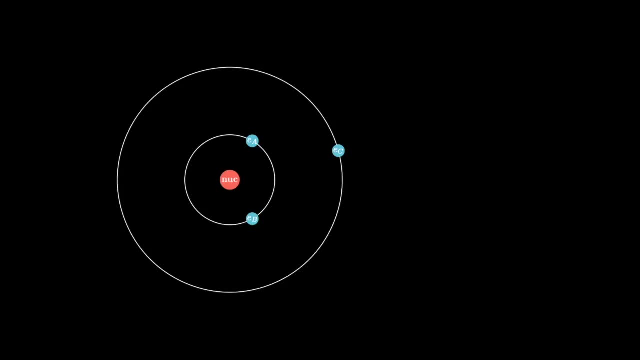 This is not a big problem because, regardless of how much I like to talk about it, spin is not the only quantum number. In this case, at least one of the electrons will have a different energy level written as the quantum number N. This will be a new variable in the function for the coefficients. 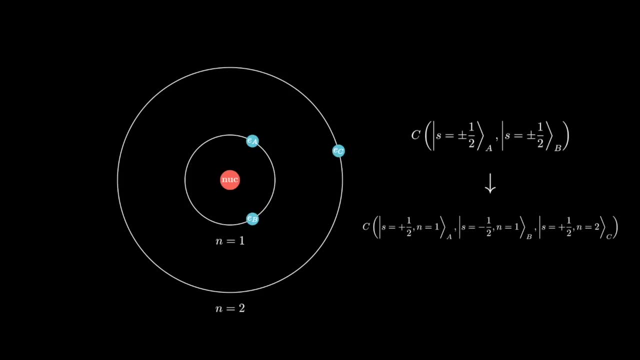 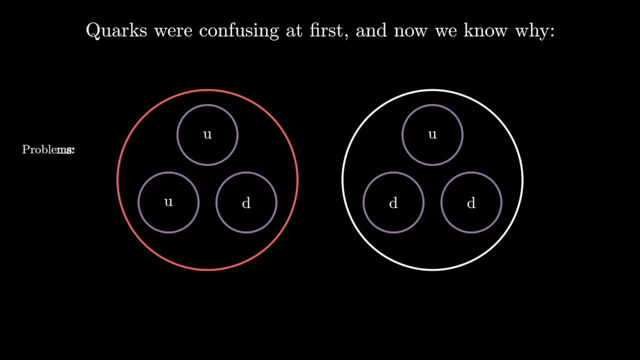 and it will take the responsibility of making the wavefunction anti-symmetric. If you remember your chemistry classes, this is the reason why you can only have twelve electrons in each energy level. Now you are finally ready. Here is why quarks were so confusing at first. 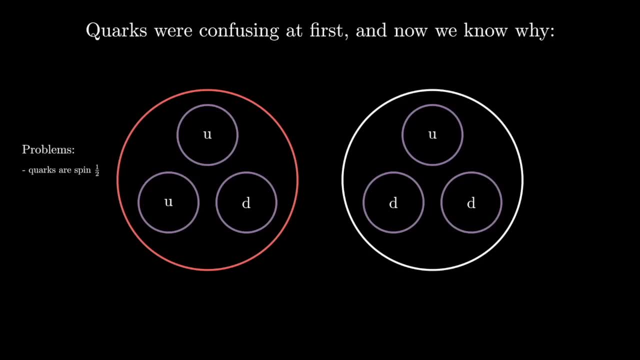 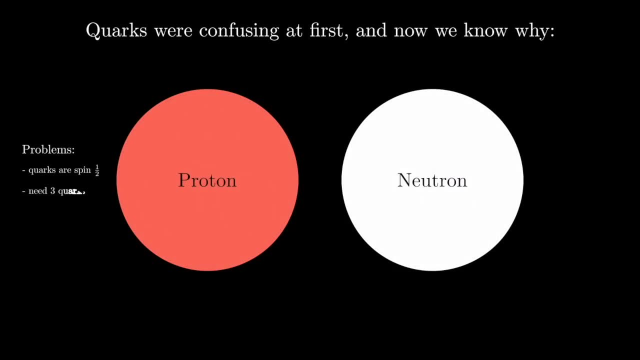 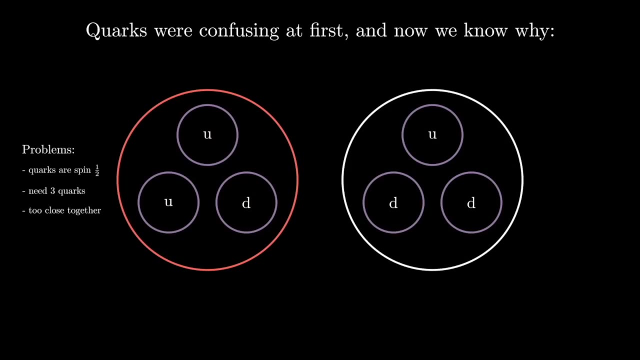 Quarks also have spin with a magnitude of one-half, and yet you need three of them to make protons and neutrons, which means spin cannot make them anti-symmetric And they are too close together to have different energy levels, so how can they possibly be? 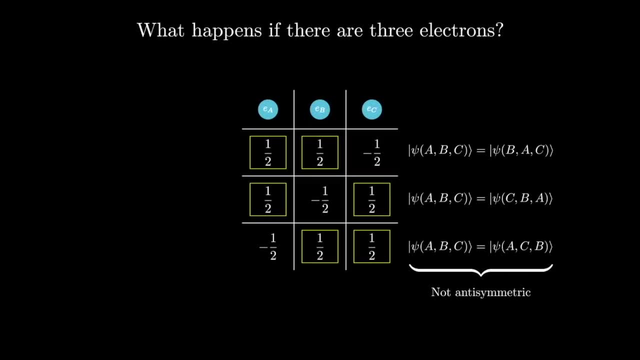 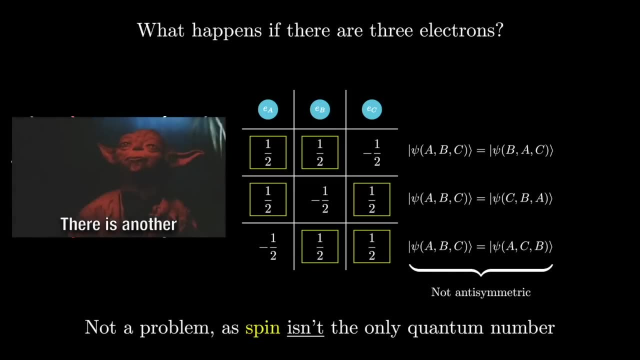 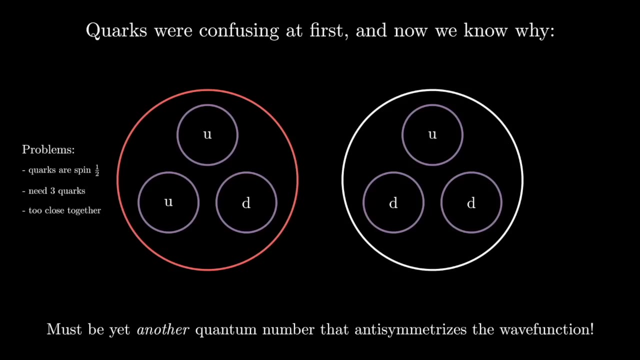 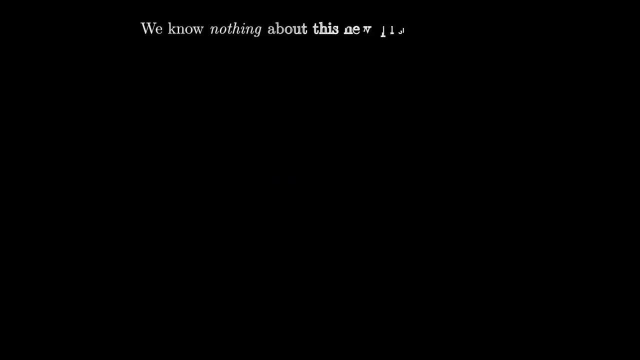 anti-symmetric. Regardless of how much I like to talk about it, spin is not the only quantum number. That's it. There must exist yet another quantum number making the wavefunction anti-symmetric. Part 2. Color charge. At this point we know nothing about this new quantum number, but we can deduce how. 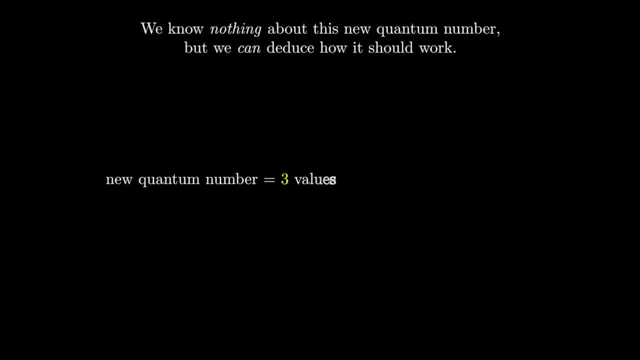 it should work. We know it needs to have a value of one. We needed to know at least three different values, one for each quark, and we can represent them as vectors from the get-go: 1 0 0,, 0 1 0 and 0 0 1.. 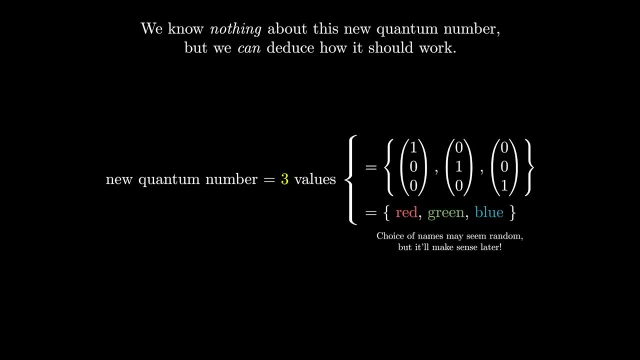 But it will be useful to give them names: Red, green and blue. These names may seem very random now, but they come from a metaphor that will make a lot of sense when we get to it. Let's say we have a proton made of three quarks: q1, q2 and q3. 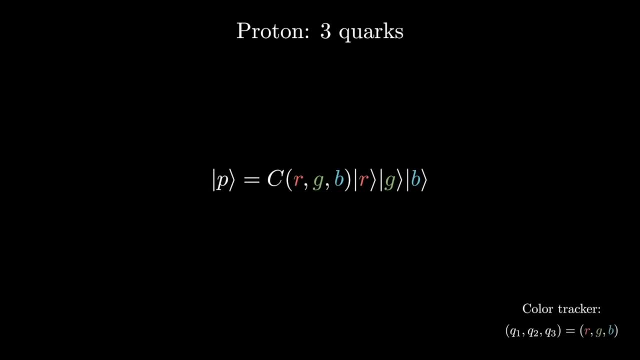 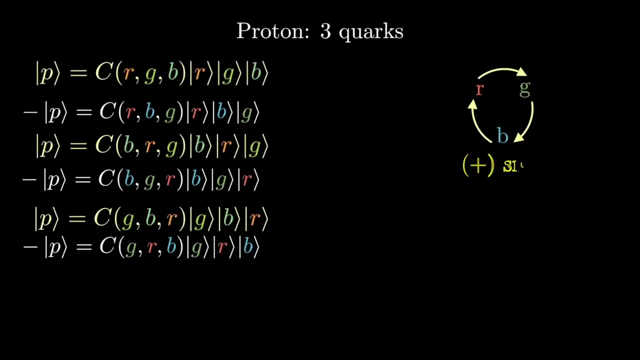 this property we are calling color. you know that if you switch the color of any two quarks, the wave function should get a minus sign. by testing more and more combinations we can start to see a pattern. it is like a cycle. if the order of the colors flows with the cycle, then the whole thing is positive, but if it flows against, 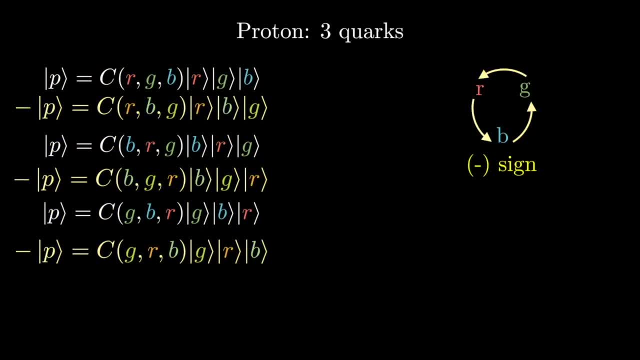 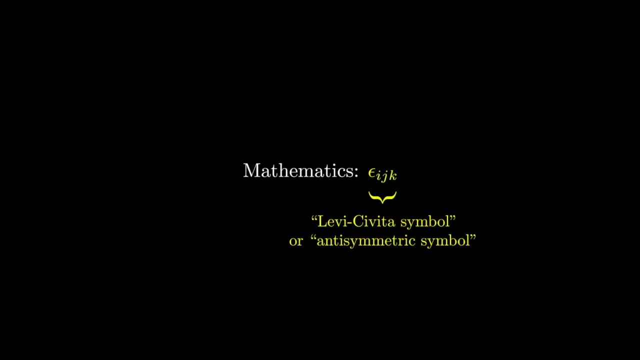 it, then it is negative. this is the color cycle, and it will be very important. turns out that mathematicians have used an object with this property for a long time. they call it the levy chivita symbol, also known as the anti-symmetric symbol. we can write the wave function of a proton. 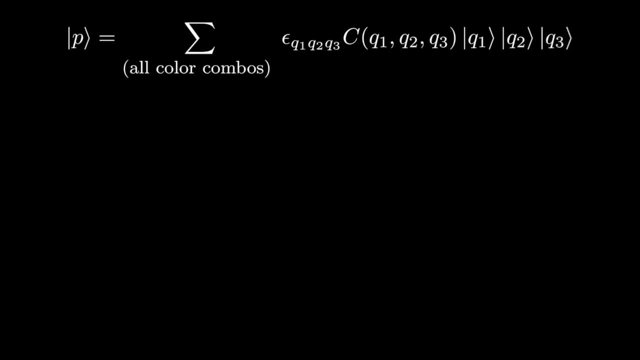 using these color states and the levy chivita symbol. like this: in each case, the levy chivita symbol will be one if the colors flow with the cycle, minus one if they flow against it, and zero in all other cases, like if one of them is repeated. 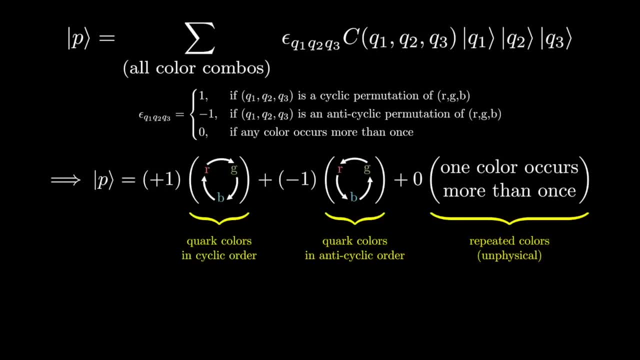 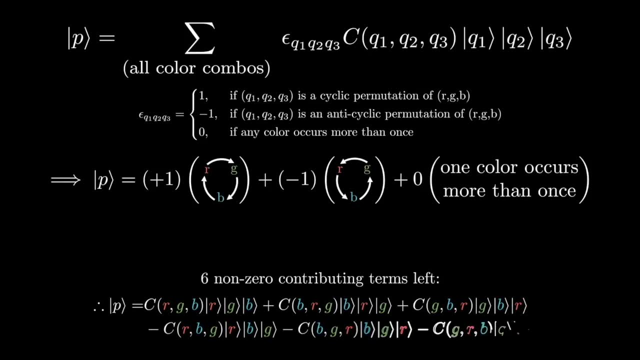 or something. after removing all the outcomes that end up with zero probability, we end up with only six. notice how, if you switch the order of two colors in one outcome, you will find another one with that order of colors but the opposite sign. part three, white, is color neutral. 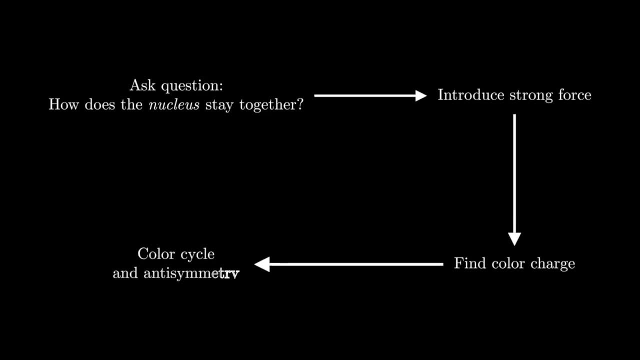 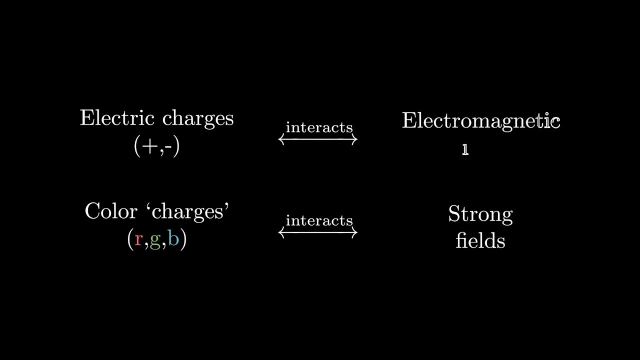 we got carried away with anti-symmetry, but remember that the whole point was to figure out how the nucleus of an atom stays together, and maybe we just figured it out. in the same way that electric charge interacts with electromagnetic fields, this new color charge interacts with strong fields each. 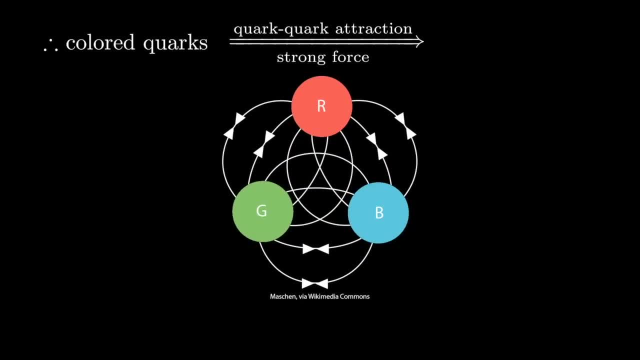 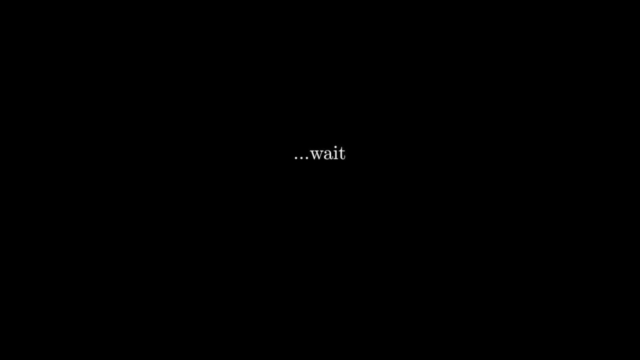 quark must be attracting the other two, and this is how they form protons and neutrons. but wait, no, something just plainly makes no sense here. if this force is so strong and if it interacts with all protons and neutrons, why is this the first you are hearing about it? shouldn't you see it everywhere in your 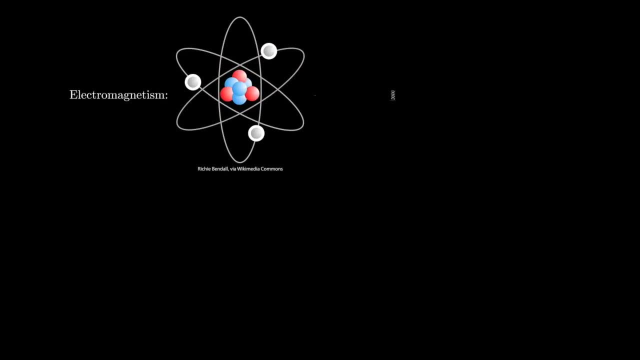 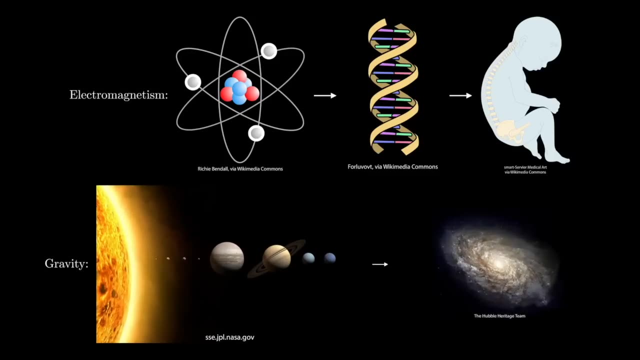 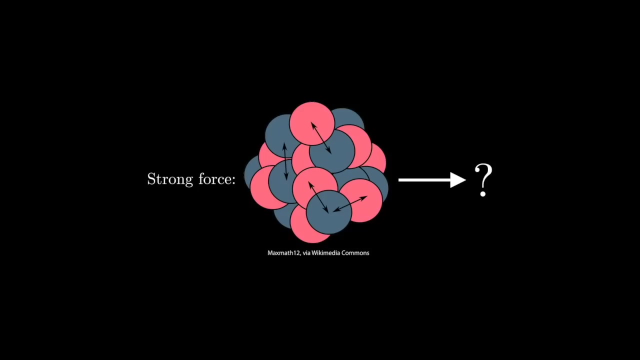 everyday life. i mean. electromagnetism forms molecules which form cells and living creatures like us. gravity forms planets, stars and galaxies, but the strong force seems to stop forming things at scale of atomic nuclei. at larger distances it seemingly disappears. to understand what's going on, we could try to find the formula that describes the attraction between color charges, the equivalent. 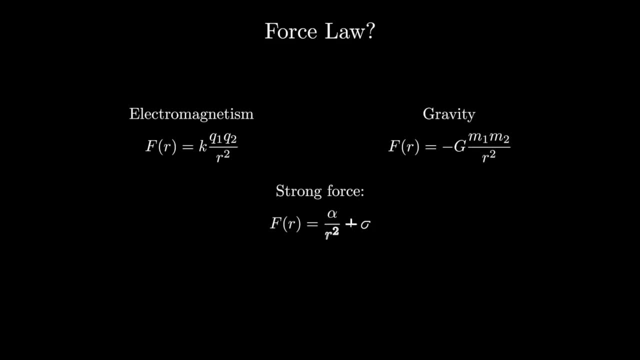 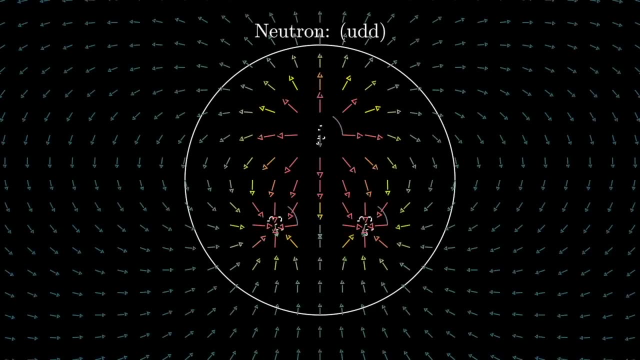 of newton or column loss, and other scientists certainly did that. but let's take another approach. let's look at neutrons. neutrons are made of two down quarks with a charge of minus one third and one of quark with a charge of two thirds. 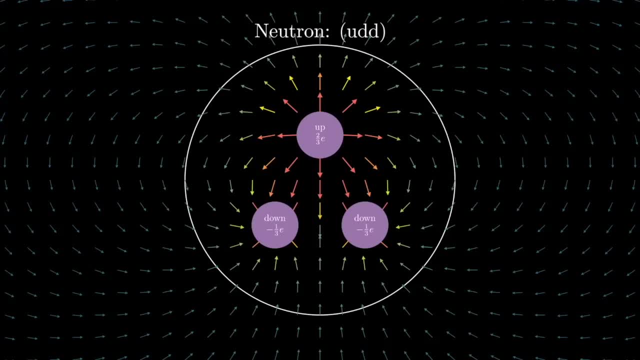 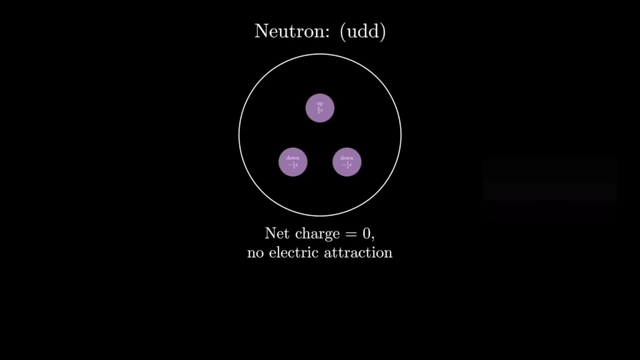 At short distances each of those quarks can feel electrical attraction, but at long distances the effect of each quark cancels out because their charges add up to zero and this makes the neutron well neutral and immune to electrical attraction. 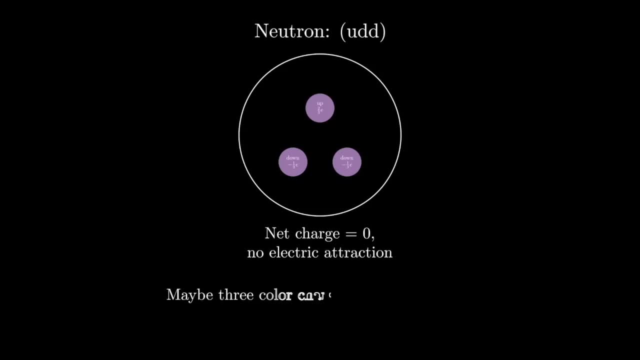 The ace of the particle world. Maybe having three different color charges acts in a similar way. Maybe at short distances each quark feels the strong force and this is how they form protons, neutrons and atomic nuclei, But at long distances they cancel each other out, making protons and neutrons colorless. 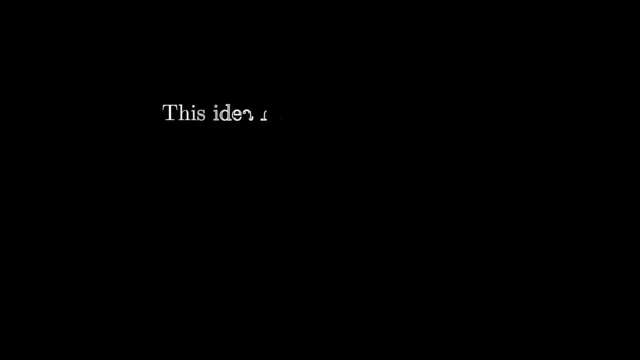 or, I guess, following this metaphor, white. We can write this idea with a simple equation: red plus blue plus green is equal to zero, But this means that red should be equal to minus green minus blue, and the same goes for all the other quarks. 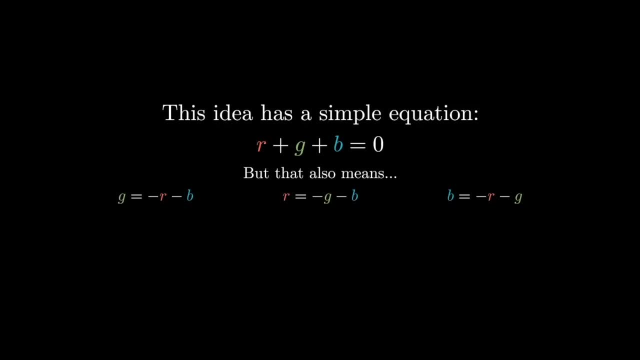 Each one is equal to having the opposite of the other two, Which is weird. I mean, for starters, what even is the physical meaning of a negative color charge? Well, just like there are positive and negative electric charges, there are positive and negative. 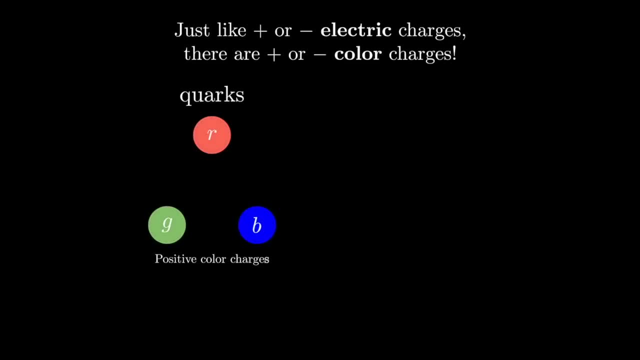 color charges. Quarks only have positive color charges, but anti-quarks, the antimatter versions of quarks, have only negative color charges And, of course, minus red, minus blue, minus green is equal to zero. Again, each negative color charge is equal to having the opposite of the other two. 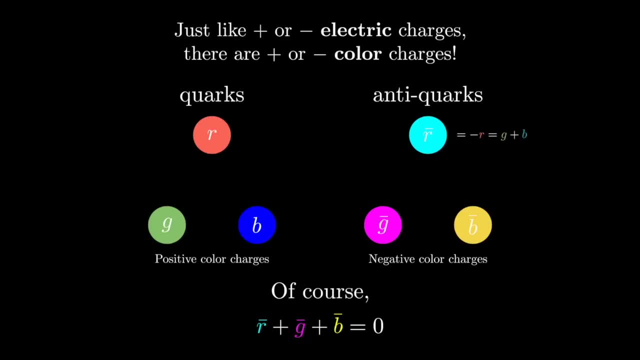 For example, anti-red is equal to green plus blue. It's perfectly natural if this sounds ABSOLUTELY BUNKERS. That was my first impression when I learned about this, But if you find this reasonable and even familiar, then you are probably a photographer. 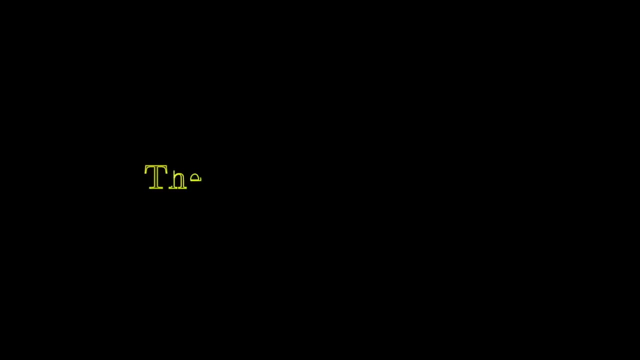 and you are probably a photographer Or a graphic designer. Part 3.5: The RGB Color Space. RGB stands for Red, Green, Blue, and it is the system used to show colors in screens. Each pixel is made of three tiny LEDs: one is red, the other is green and the last one. 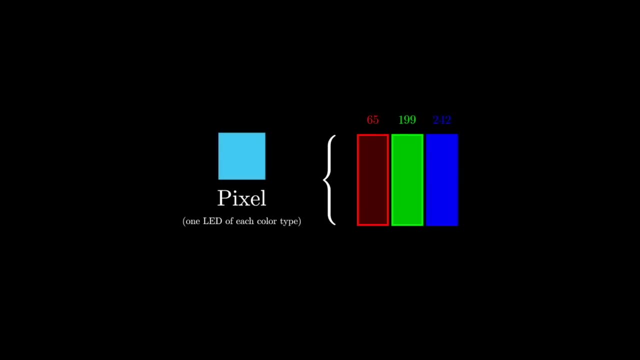 is blue. The screen can make each LED shine with different intensities, ranging from being completely off, which is called zero, to shining as bright as the device allows, which is called 255. for engineering reasons, The combination of these different intensities can give us the illusion of many different 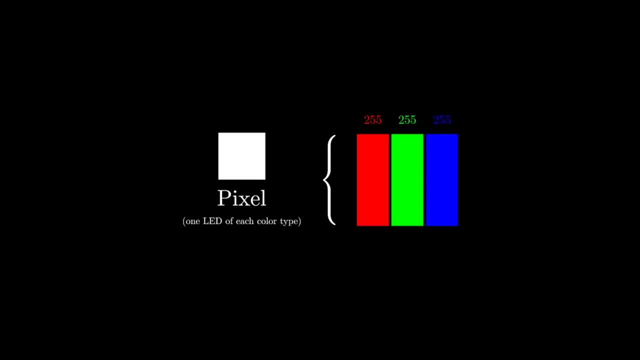 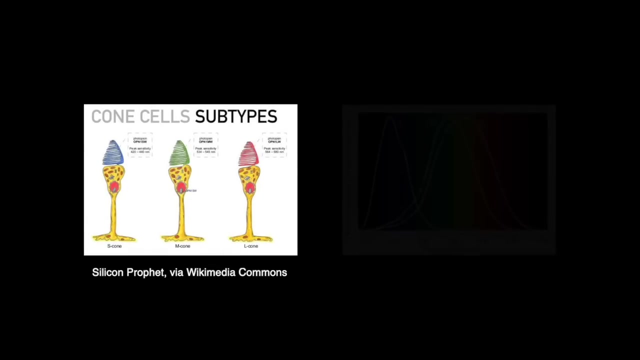 colors. For example, if all three LEDs are at their maximum intensities, we will see it as white, But then, if we turn off the blue LED, we will see it as yellow. This happens because we have three kinds of color receptor cells in our eyes. They are tuned to trigger at specific frequencies of light, But there is some overlap. For example, the cells that detect red and green light are both triggered by yellow light, So when we see red and green at the same time, our brains assume we are just seeing yellow. 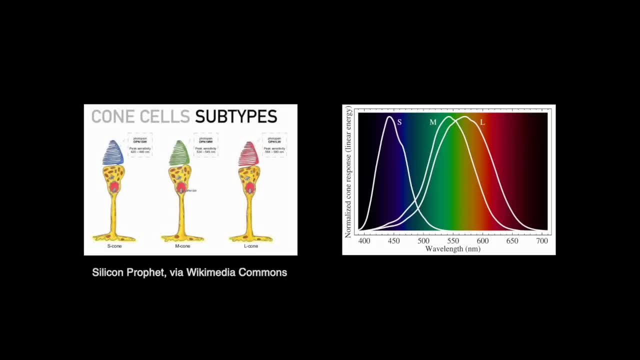 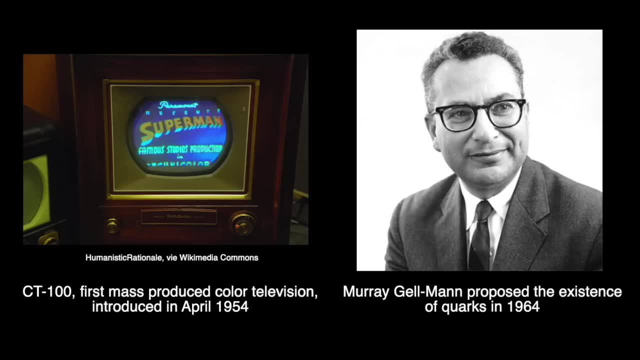 light, even if there is no yellow light reaching our eyes. This system was first invented for color televisions in the 1960s. And what do you know? these discoveries about? quarks were being made in the 1960s. Just like we have done a couple of times now. 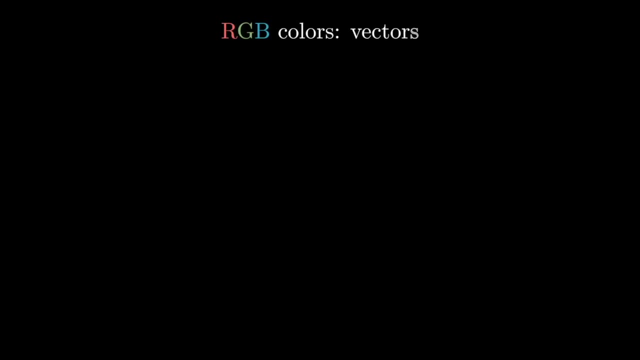 We will visualize colors in the RGB system as vectors. For example, white will be 255, 255, 255, and yellow will be 255, 255, 0.. But wait a second. The vector 00255 is blue, right. 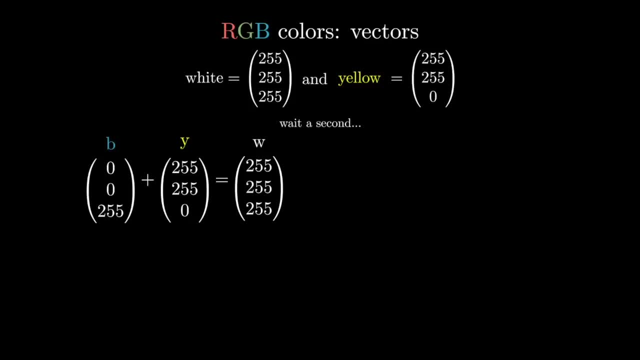 And if we add this yellow vector, then we get white. Huh, In a sense It's like they cancelled each other out. In this system, yellow is the opposite of blue, But yellow is made of red and green. We can do the same for the other colors. 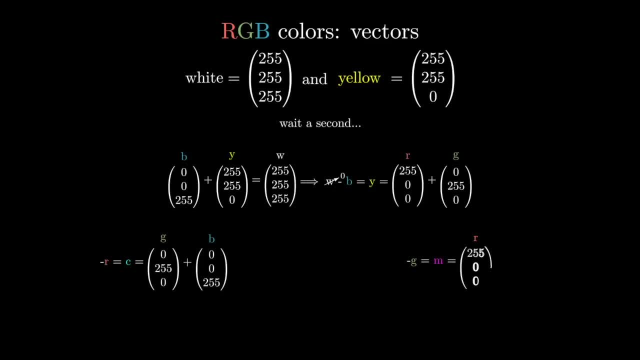 Green and blue make cyan, which is the opposite of red, while red and blue make magenta, which is the opposite of green. Can you see the similarities? The mathematics used in the RGB system are the exact same mathematics, followed by the color charges of the strong force. 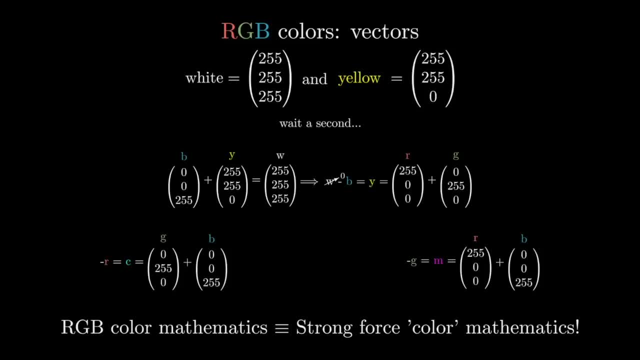 And this coincidence is the reason the color charges are called color charges in the first place. But I know something is nagging you at the back of your head: How come two completely different things ended up being described by such similar mathematics? You'll figure it out soon in the next section, I promise. 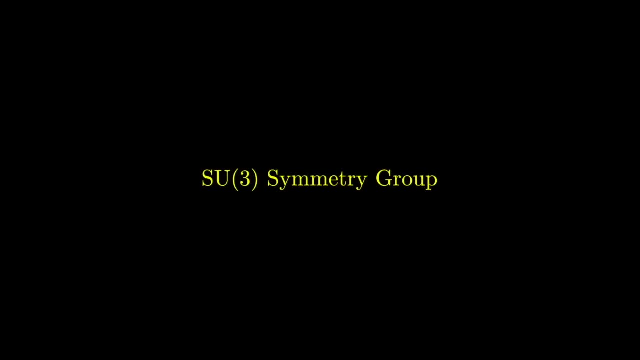 Part 4.. SU3, This is all insanely cool, isn't it? Using Pauli's exclusion principle, You deduce the exact same thing. You deduce the existence of a new property of matter, And you use the fact that it cancels out at large distances to deduce that it follows. 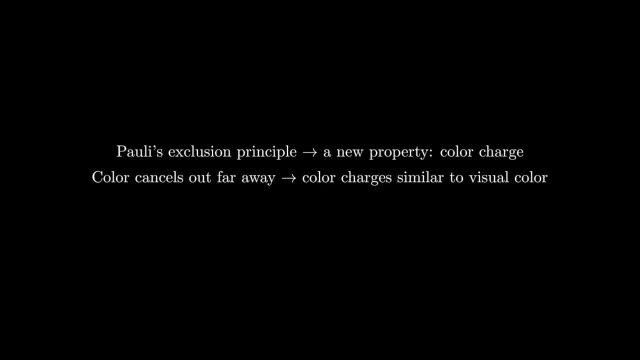 the same mathematics as the RGB system, But there is still one problem: Magnetism. Even if protons and neutrons have zero color, even if they are white, they could still interact with the strong force. The easiest way to think about this is to look at neutrons again. 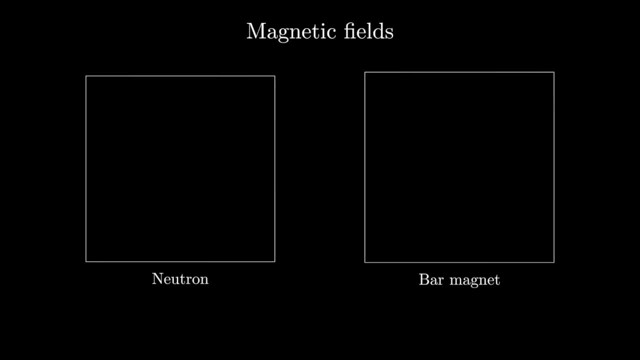 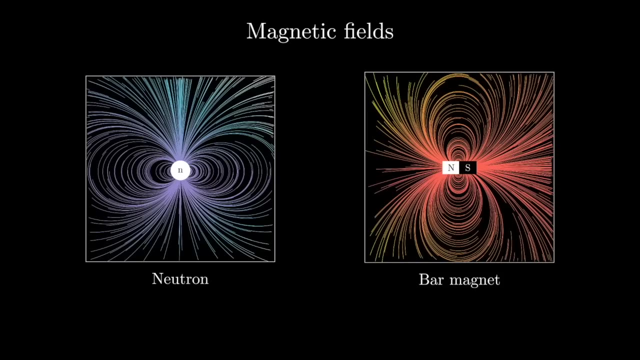 They might be electrically neutral, but they still have magnetic fields. You can see this with the magnets in your fridge. They don't shock you when you touch them because they have neutral electric charge, But they can still interact with the magnetic part of the electromagnetic force. 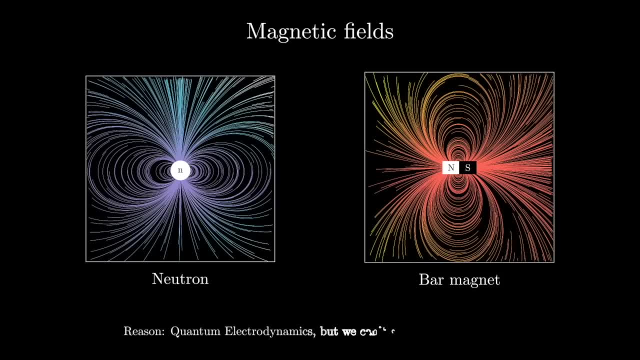 And quite strongly. The reason this happens lies deep in quantum electrodynamics. But, in summary, it happens because the electromagnetic force is transmitted using photons, And photons are neutral. They do not have electric charge. If photons have electric charge, They have electromagnetic field. 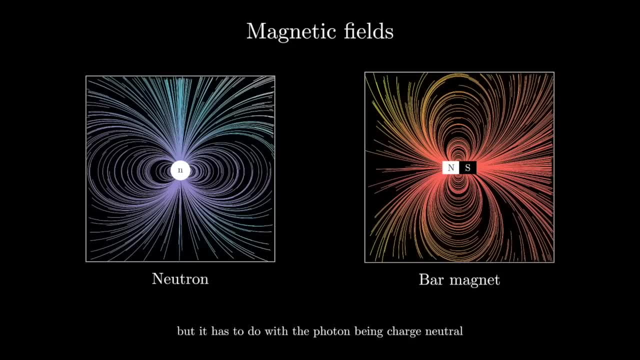 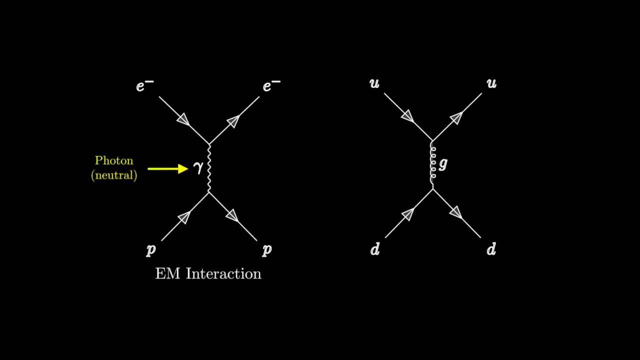 Then there would be no magnetism. The strong force is transmitted using particles called gluons. They have this name because they keep the nucleus glued together. Get it No, Whatever I mean. it's not like it's my joke, I didn't come up with it. 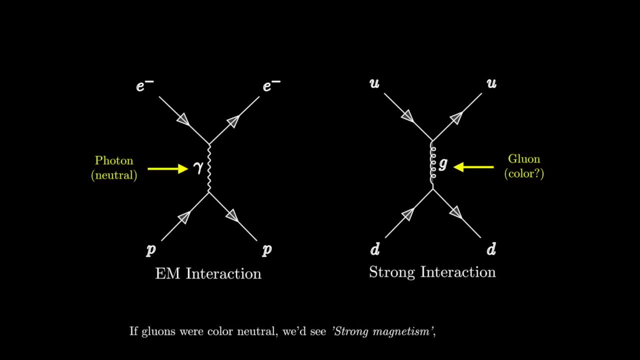 Anyway, If gluons were neutral like photons, then there would be a sort of strong magnetism. But we see nothing like that in nature, Which means gluons must not be neutral, They must be carrying Color charge. This is one of the cool differences between math and physics. In physics you can just say, hmm, I looked really hard for something and I couldn't find it, So it doesn't exist. But in math, people can fail to find something for 4,000 years and they will still not accept. 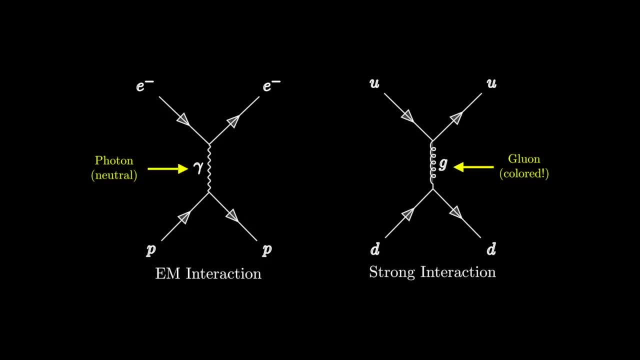 that it doesn't exist, Just like my soulmate- I know she's out there Going back to gluons. Consider this Feynman diagram. Here we have two op quarks. The first one is a magnet. The second one is a magnet. 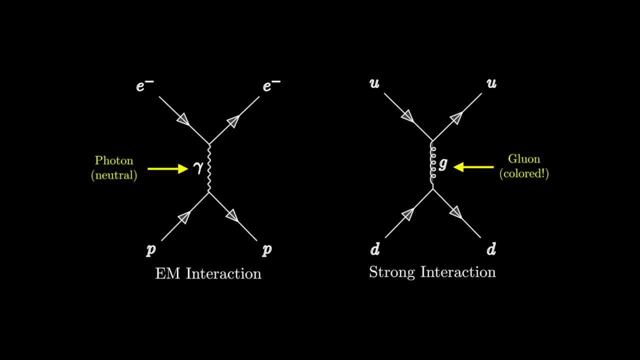 The third one is a magnet. The fourth one is a magnet. The fifth one is a magnet. The sixth one is a magnet. The sixth one is a magnet. The seventh one is a magnet. The sixth one is a magnet. The sixth one is a magnet. 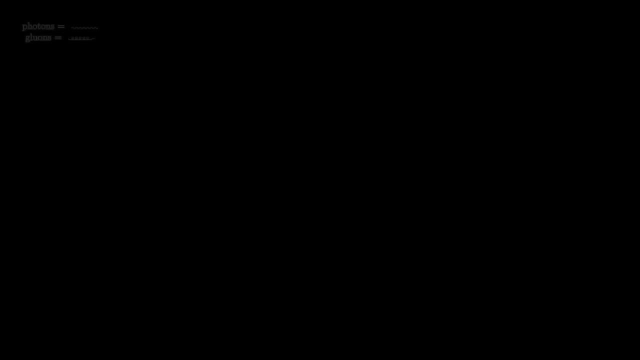 And they interact through the strong force. by exchanging a gluon, Maybe this green quark emitted its green charge and it was absorbed by this other quark. However, a quark cannot remain colorless again. that would produce strong magnetism. 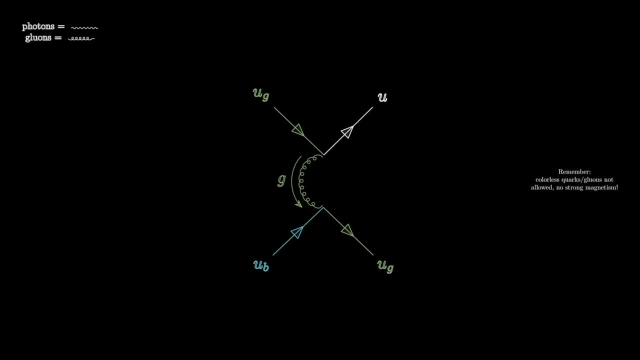 To fix this. maybe this blue quark also has the green charge that would be available in the right-hand side of the diagram- emitted its glue charge and in this way they switched colors. At first it looks like they emitted two gluons because two kinds of color charge were exchanged, but 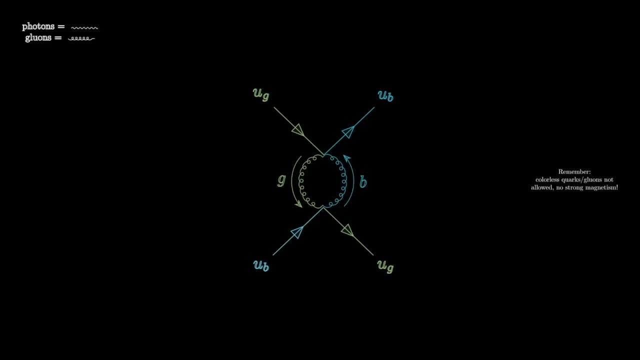 since this was a single interaction, they must have exchanged a single gluon and that gluon must have been carrying two color charges. In fact, gluons always carry two color charges. Let me show you. Maybe this green quark became blue and to ensure that a total amount of color charge remained the same, it emitted a. 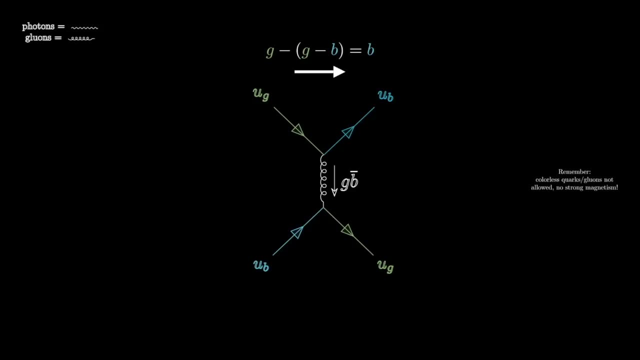 gluon carrying two color charges- green and anti-blue, because when we subtract the color charge of the gluon from the color charge of the quark it adds up to blue. Then the blue quark absorbed the emitted gluon: blue and anti-blue. 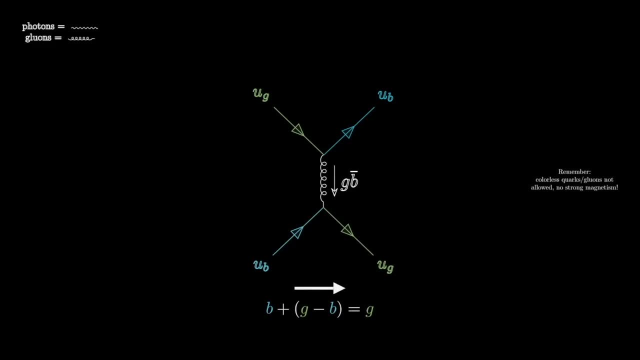 cancelled out and this quark disappeared. The green quark was left only with the green charge and in this way they switched colors. Or maybe it happened the other way around. Maybe the blue quark emitted a gluon carrying blue and anti-green? Hmm, how can we know? That's the fun part. 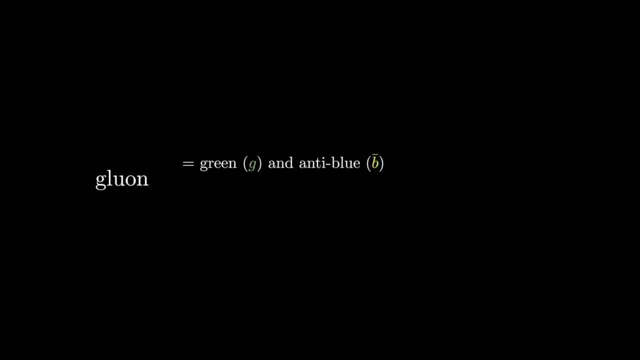 You don't. We must always consider gluons as the two possibilities they could have been. They too are vectors of probabilities. And now a question starts forming in your mind. It may be a little hard to express, so let me help you out. 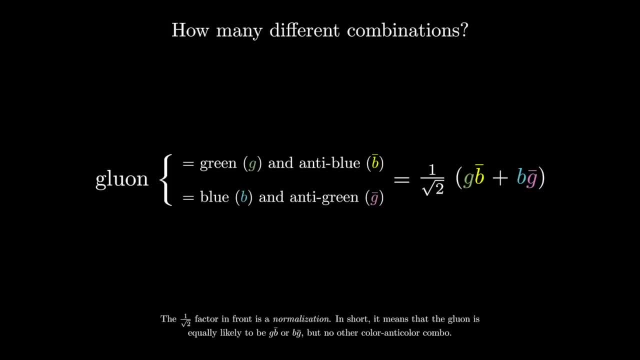 How many different combinations do we need to create all possible gluons? Or, in terms of linear algebra, how many linearly independent combinations of gluons are there? This is a very important question. It will tie everything together once we solve it. But to solve it we must go back to spin. I know it always. 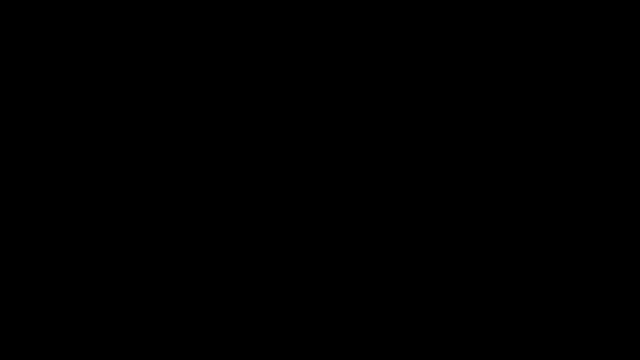 goes back to spin Part 4.5: Singlets and triplets. Ok, I know this video has been long enough, but this is the home stretch. We can do it. Consider a hydrogen atom, a proton and an electron. Once again, there are four possible. 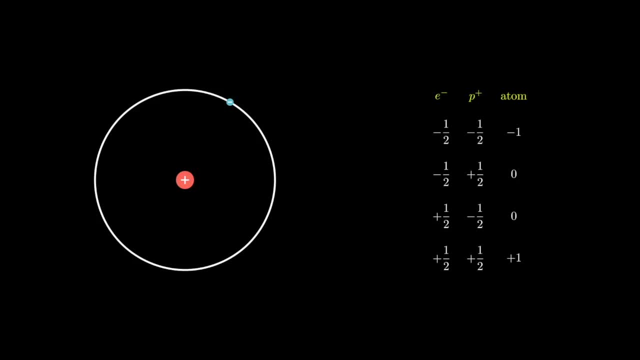 spin combinations, but since there are many differences between them, they are allowed to have the same spin. Let's imagine both of them have a spin of minus one half. Then the total spin of the atom is minus one. Next, we shoot a photon with spin one at this atom. It is absorbed by either the 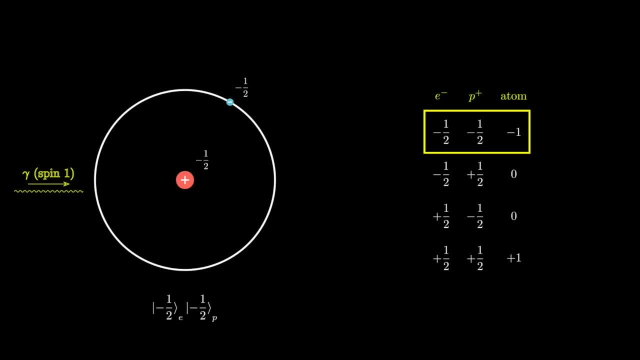 electron or the proton. We don't know which one absorb it, but we know the action of this photon is to change spin from minus one half to one half. Remember From the beginning of the video. Once again, we can represent this as a combination. 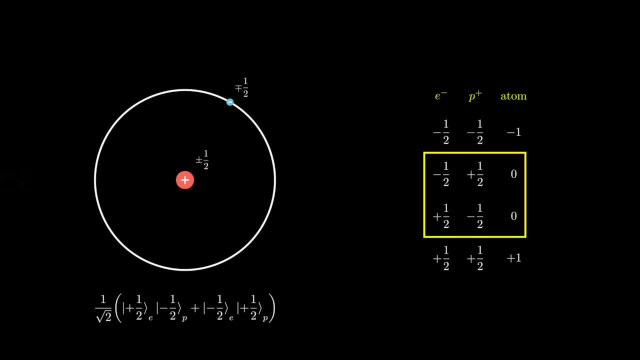 of two possibilities: One in which the electron absorbed the proton and one in which the proton did Regardless. in either case, the total spin of the atom is 0.. Next we shoot another photon with spin 1.. Once again, we don't know which one absorbed it, but we know it had to be whichever particle. 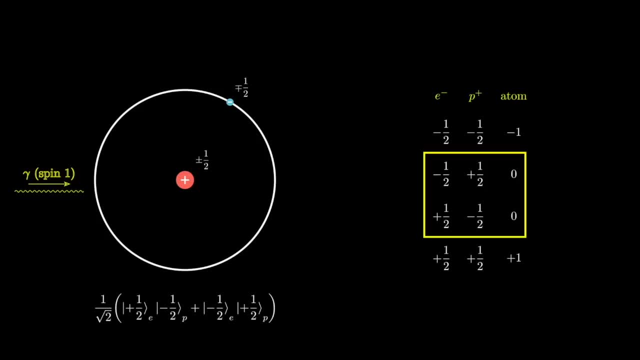 had a spin of minus one half, because their spin cannot go above one half. We can apply the action of the photon to both states and, what do you know, they end up being identical. so we can add them up and the total spin is 1.. 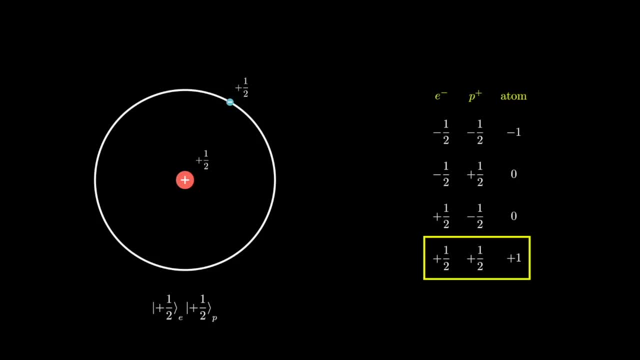 In the end, this atom has a spin with a magnitude of 1, it is a boson, and for that reason it is free to move up and down between these three states Together. we call them a triplet state, But what I want you to notice here is that the photon is secondary. 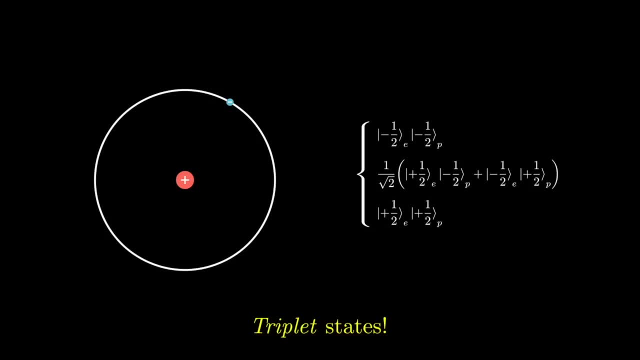 Its action is what really matters. These three states are related to each other by the action of going up or down in spin. Remember that. Let's go back to when the spin was 0.. What if this plus sign was a magnitude of 1?? 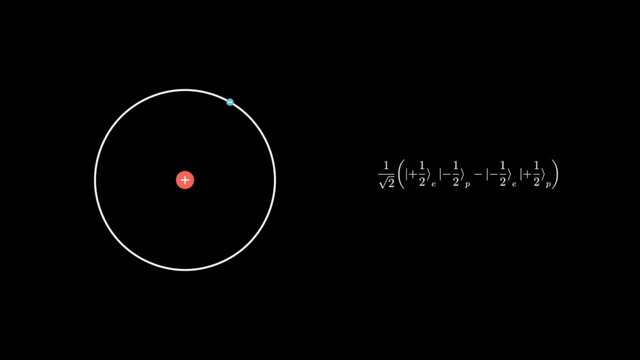 Well, if we apply the action of going up, we end up with two equal states, just like before. but now they don't add up, they cancel out. And yet the wavefunction cannot be 0, because the atom cannot just stop existing. 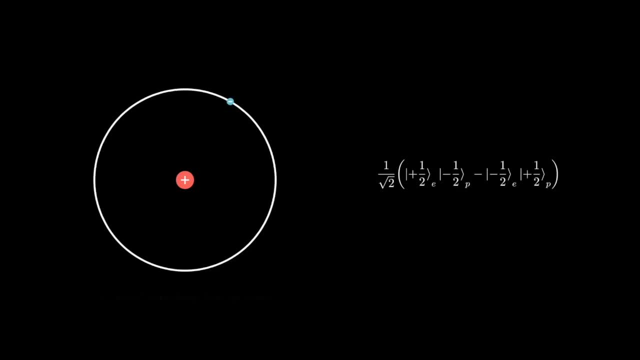 Instead, if this atom absorbed a photon, it will simply move the electron farther or closer to the proton, but the spin state will remain the same. In other words, This atom is behaving like a boson, but a boson with a spin magnitude of 0, and for 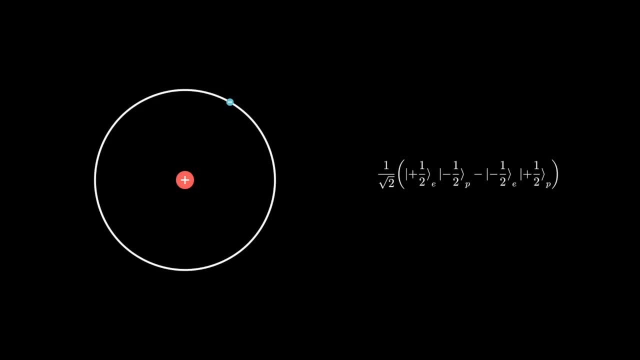 that reason, it only has one allowed state: 0.. This is called a singlet state. Finally, finally, we are ready. Everything in the video has been leading up to what comes next. Let's look at one possible gluon. This one is carrying either red anti-blue or blue anti-red. 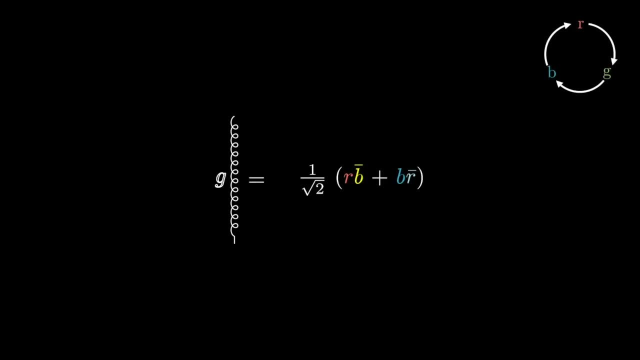 Now, If we go down the color cycle, we can see that before red is blue and before blue is green. For that reason, if we went down the color cycle, we would find the state blue anti-green plus green anti-blue. Next, if we continue going down, we will find the state green anti-red plus red anti-green. 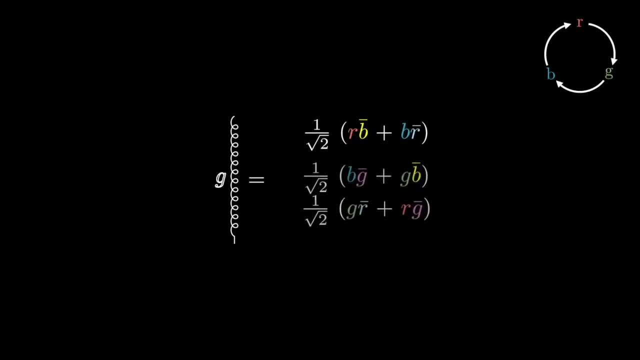 Here we have three states with a sort of relationship between them regarding going up or down. This is analogous to the third state. This is analogous to the third state. This is analogous to the triplet state from before. As you can imagine, this means we should have a state analogous to the singlet blue, anti-green. 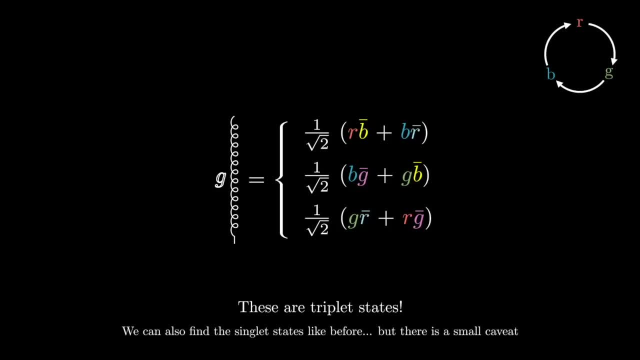 minus green, anti-blue. However, there's a small caveat here. In the case of spin, one of the states has to be flipped to be negative, right. Well, in this case we do that, but we also must flip the whole thing around the complex. 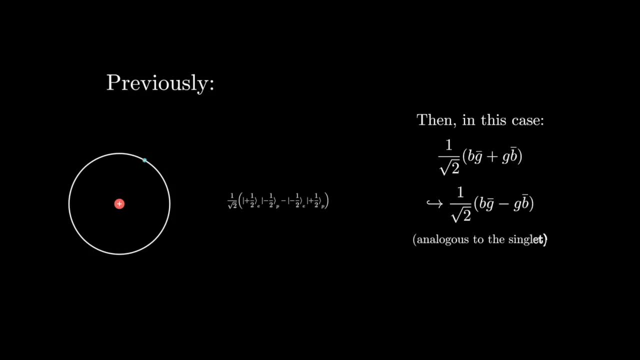 plane by multiplying everything by negative. i Sigh. I would love to go into detail about why we have to do this, but this is one of those things that should be its own video. Hopefully, the notion that we have to flip the vector in more ways than one is enough. 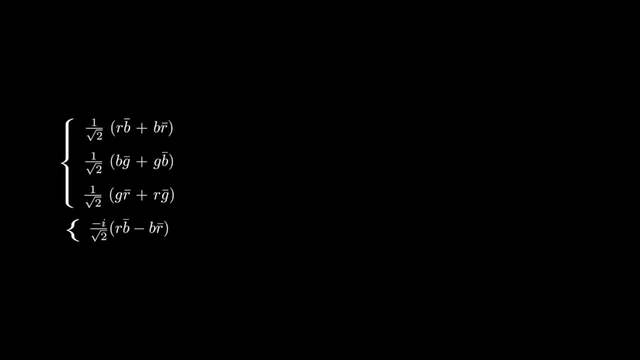 for now. Anyway, we have a triplet and a singlet, just like before. but who said we were done? We can keep going down the color cycle, or up, for that matter. If we do, we are not going to find any new states. 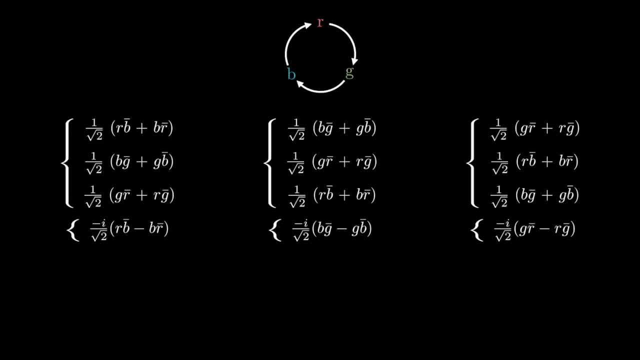 Just the same three over and over, But we do find that we can group them in three sets. Each of these sets is like a triplet, and thus it should have the corresponding singlet. Of course, these six states are not triplets and singlets exactly, but they are related. 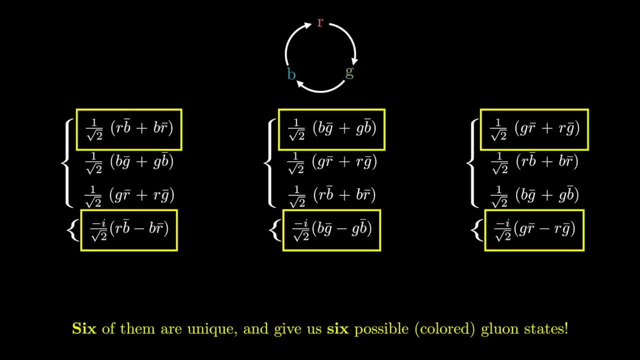 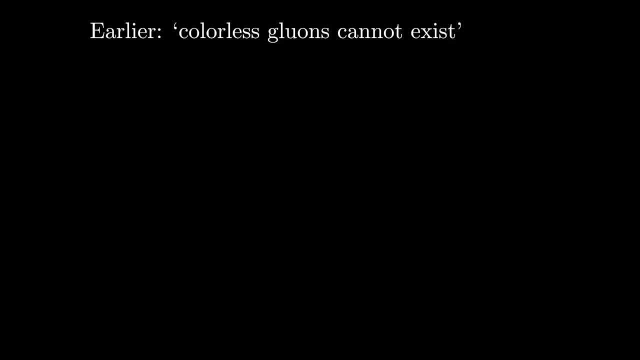 to those concepts and we will see why in a bit We are so close. Earlier I mentioned that colorless gluons must not exist to avoid strong magnetism. Now I can say more precisely that the problem would be colorless gluons that are not affected. 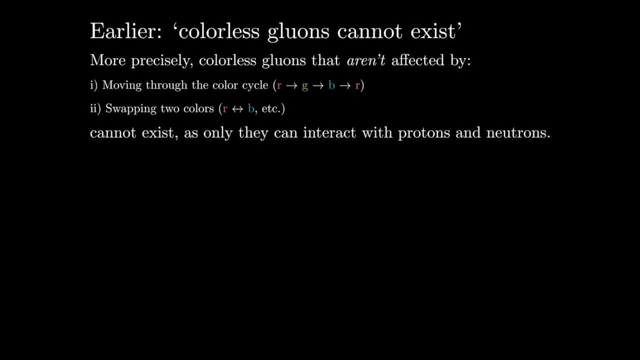 by the actions of moving through the color cycle or switching colors. Only those gluons could interact with colorless protons and neutrons. For example, one of these colorless gluons would be the symmetric state red anti-red plus blue- anti-blue. 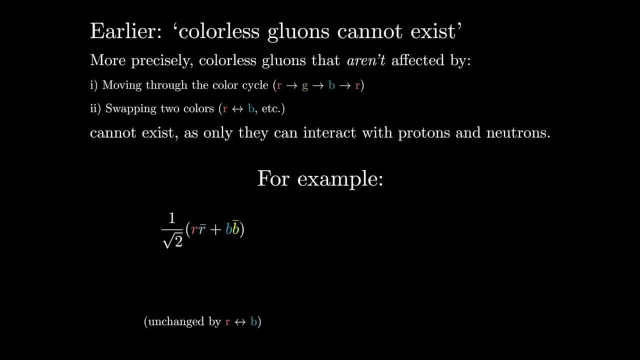 Because if we switch red and blue, it remains the same. But the worst of them all would be this one, This, This, This And this: Red anti-red plus necroprotein plus color-singlent. Red anti-red plus green anti-green plus green anti-blue. 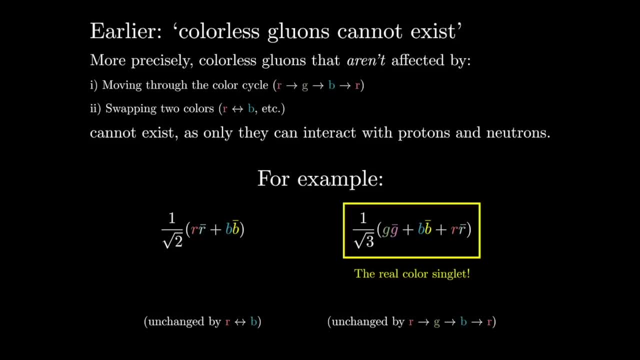 Now let's mention what some do, and we'll get that in no time: Red anti-red plus necroprotein plus blue anti-blu. No matter what actions you do to this, which direction you move through the color cycle, nor how many times, it just never changes. 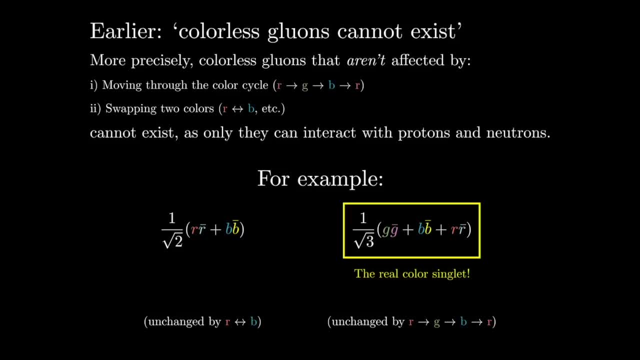 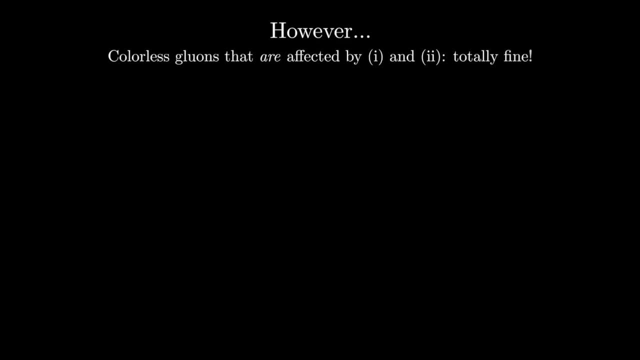 If gluons could take this state, the universe would be a very different place. However, we can totally have colorless gluons as long as they are affected by these actions. Take, for example, red anti-red, minus blue anti-blue. Ok, If we switch red and blue, we end up with an anti-symmetric state. 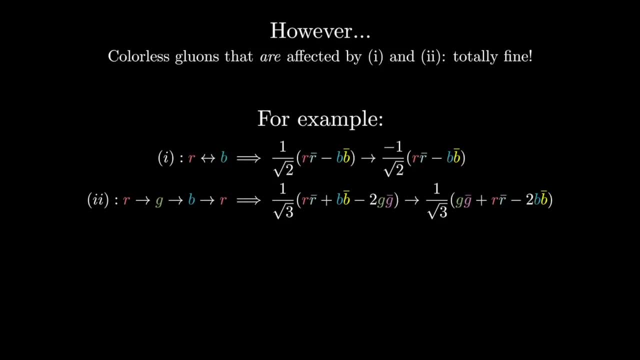 Therefore, this gluon can exist because it could not interact with colorless particles. As it happens, we can create all colorless gluons using only two of them, So we'll use this one and that one. In the end, we are left with only eight gluons. 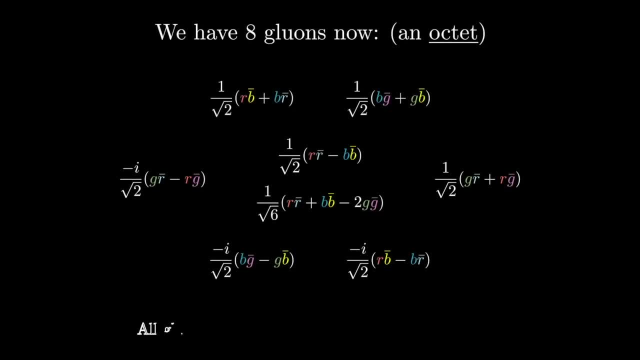 No matter what experiment we study or what process we describe, whatever gluons are involved, they can always be described as combinations of these eight gluons. But the thing is that this is not the only group of eight gluons we could use To find the other alternatives. we can once again move through the color cycle. 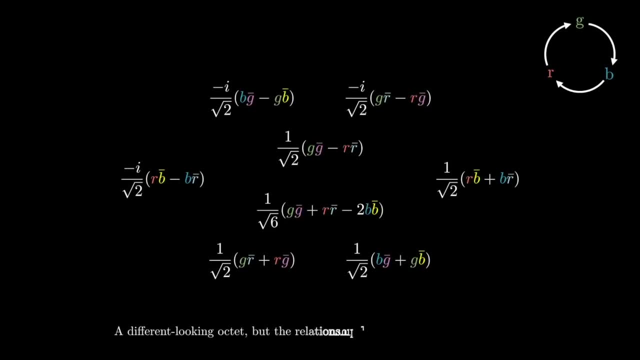 These new sets look slightly different, but the relationship between the gluons in each of them are the same every time. In other words, this set is symmetric under the action of moving through the color cycle. When we find a set that is symmetric under a certain kind of actions, we call it a group. 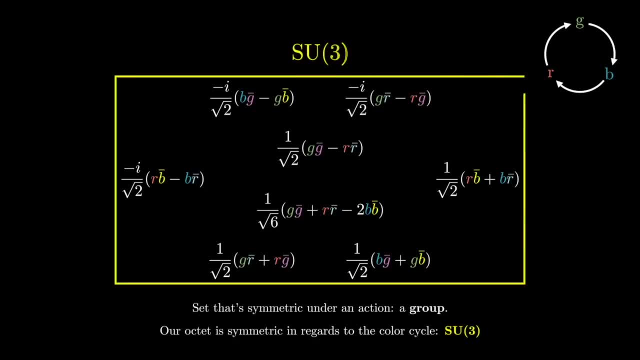 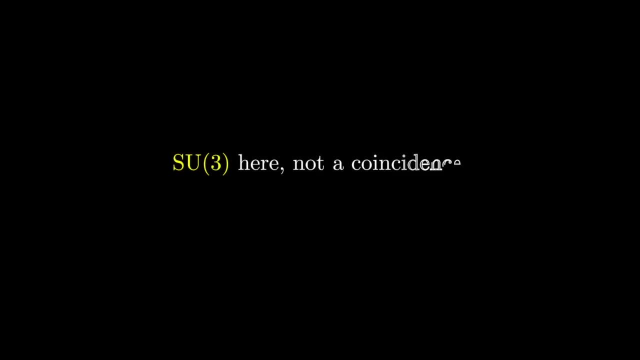 The group we found here has a name: the special unitary group of order three, But among friends they call it SU3.. The fact that we found SU3 in here is not a coincidence. Everything we've been trying to understand about the strong force is a consequence of. 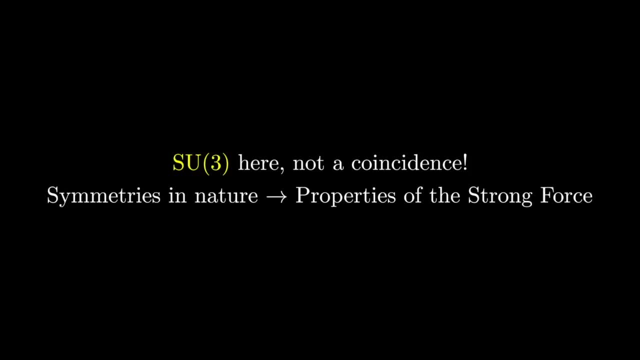 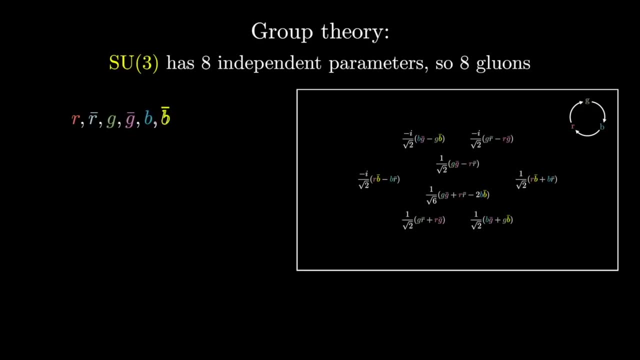 the fact that nature follows this symmetry. SU3 must be represented using eight different groups. The groups have to be eight different elements, so there have to be eight gluons. There must be a cyclic relationship between six of them, so there have to be six color. 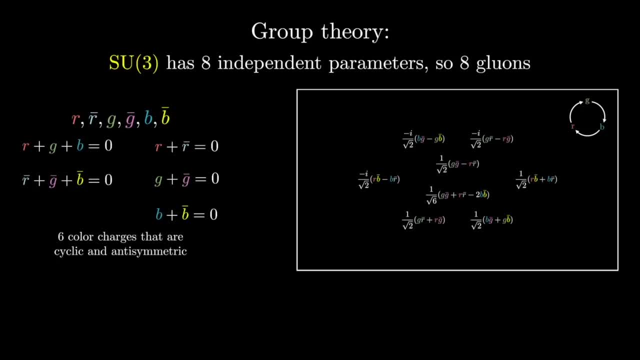 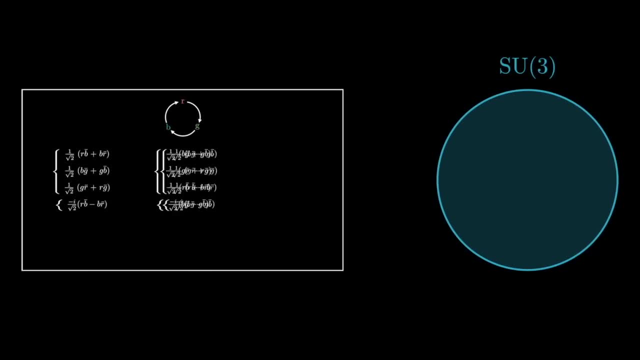 charges and they have to be antisymmetric. The other two elements have to be outside of that cycle, so the six color charges have to cancel each other out somehow. The analogs for triplets and singlets exist because SU3 contains three copies of a smaller. 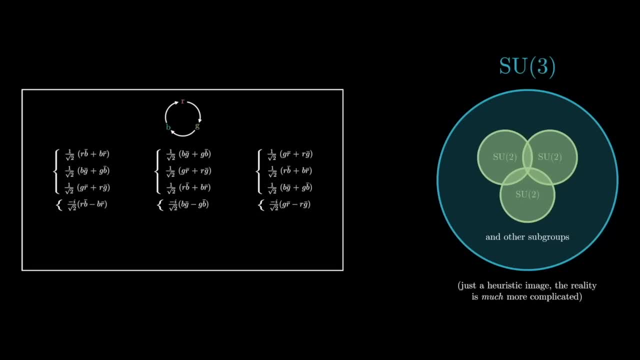 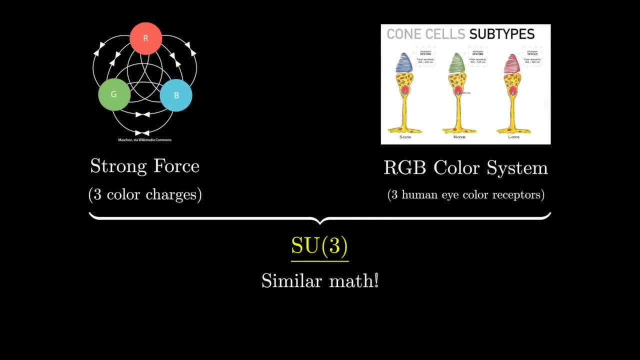 group known as SU2, and it just so happens that spin is described by SU2.. The reason It's similar math to the strong force. it's because we have three kinds of color receptors in our eyes and the combinations of those three things is also described by SU3. 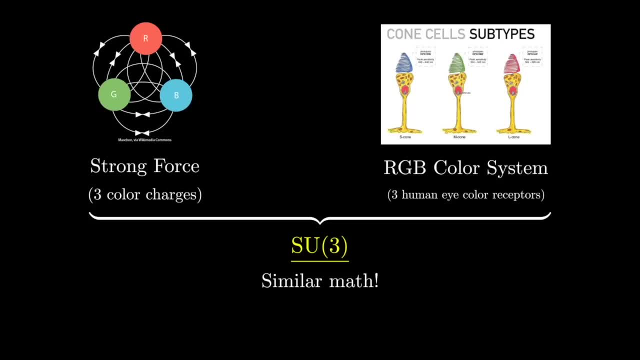 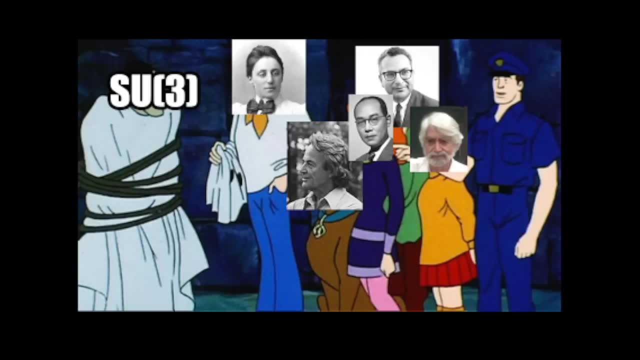 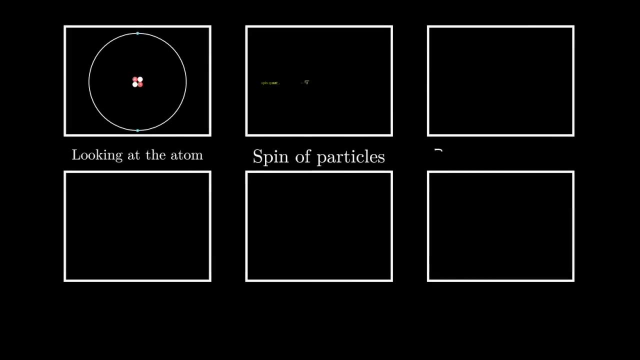 It's beautiful. It is so beautiful. It was SU3 all along and it would have gotten away with it had it not been for those meddling kids. Okay, I've calmed down now, but my point still stands. How mind-blowing is it to realize. 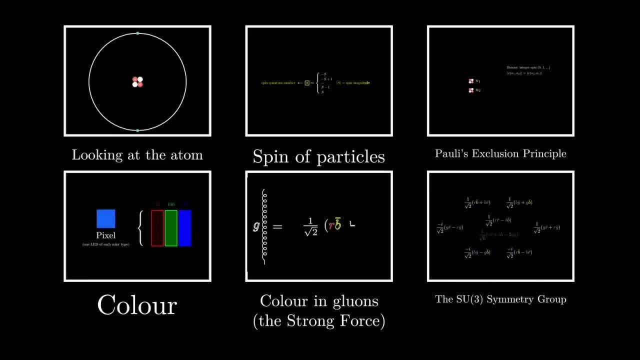 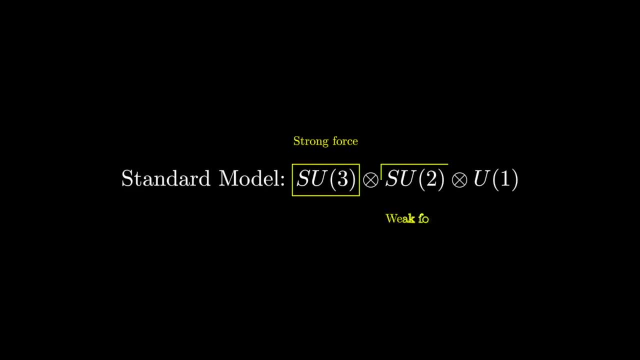 It's easy to realize that all of the properties of a force of nature are the consequence of a mathematical symmetry, a symmetry that can exist in other things, like in our eyes, by sheer coincidence. And the strong force is not the only one: electromagnetism and the weak force are the 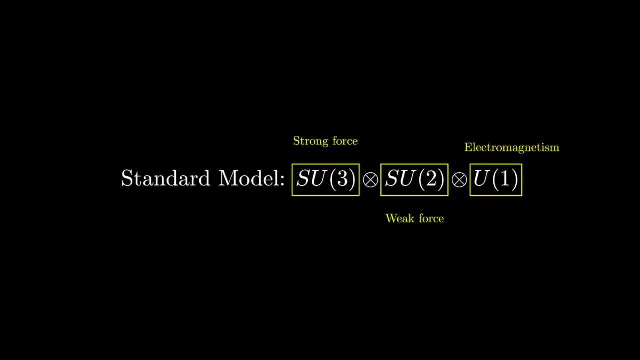 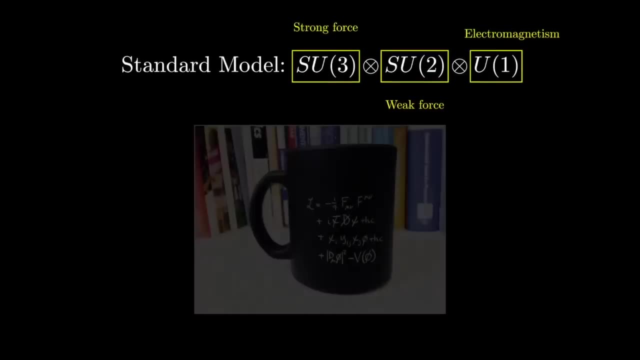 result of symmetries known as U1 and SU2.. But what about gravity? Don't mention gravity. We were having a good time. In fact, when you combine all these symmetries, you get the following: When you combine all these symmetries into a single equation, you get the standard model.